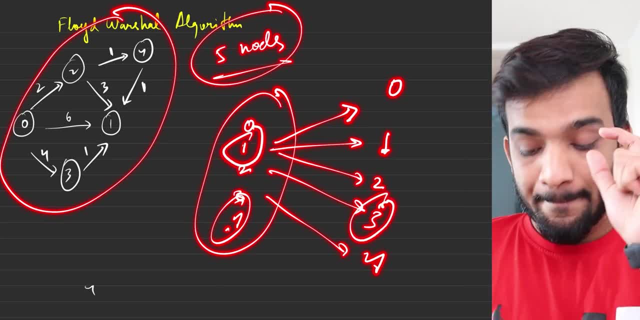 be able to tell me the shortest path to every other node over here. If I'm asking you from 4 to 1, you should be able to tell me the shortest path to every other node over here. If I'm asking you from 1 to 3, you should be knowing. So there are multiple, multiple source. so this is why this is. 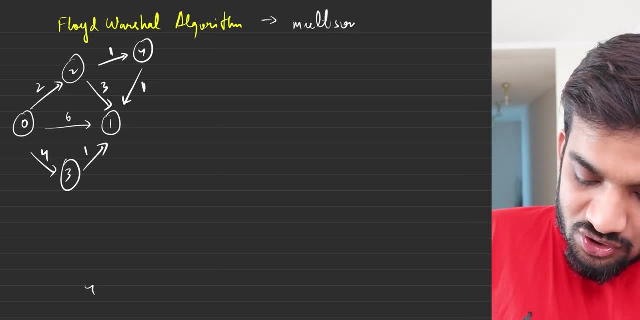 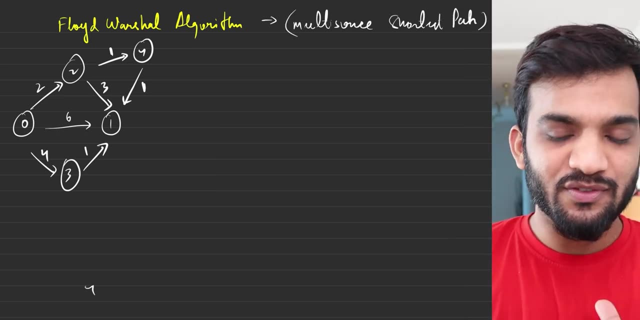 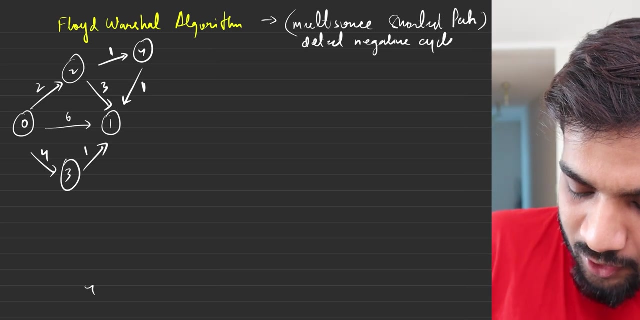 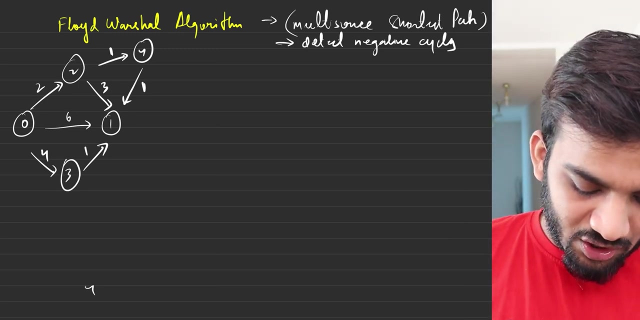 known as a multi-source shortest path algorithm. Remember this. it helps you detect negative cycles as well. helps you detect negative cycles as well. So I hope pretty much you've understood what you need to find. Now, what is the shortest path? Very simple, if I'm asking you from 0 to 1. 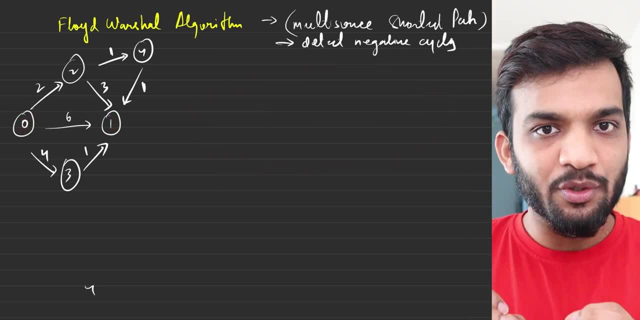 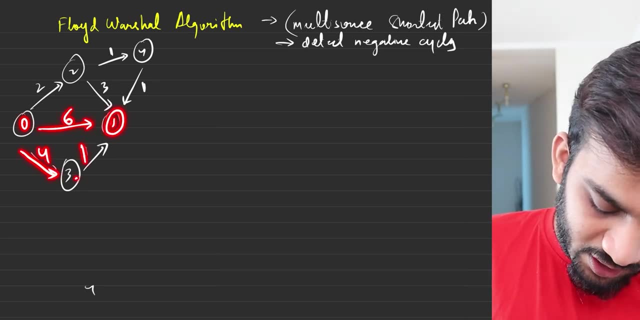 and I ask you: what is the shortest path in order to reach from 0 to 1.. So you can take multiple paths. one of the path will take you 6. you can take this path, which is going to take you 5. you can take probably this path, which is again going to take you 5, or you can take the shortest. 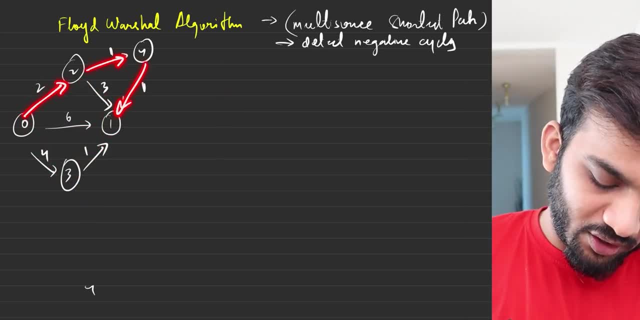 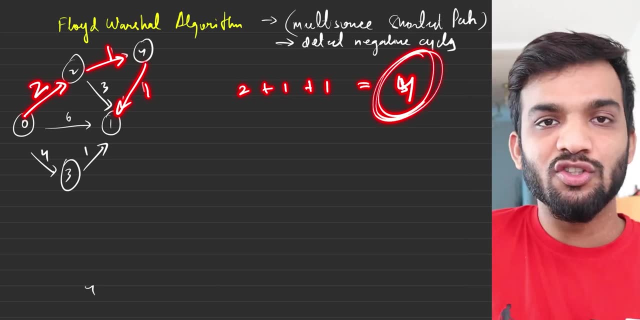 one which is: go here, go here, go here, which is going to take 2: 1, 1 which is an addition of, I think, 4 here that's the shortest path. So the shortest path from 0 to 1 is 0 to 2. 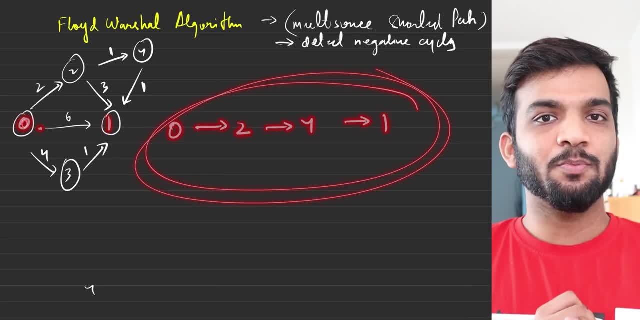 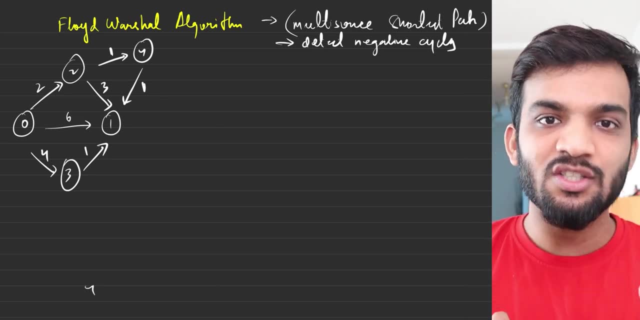 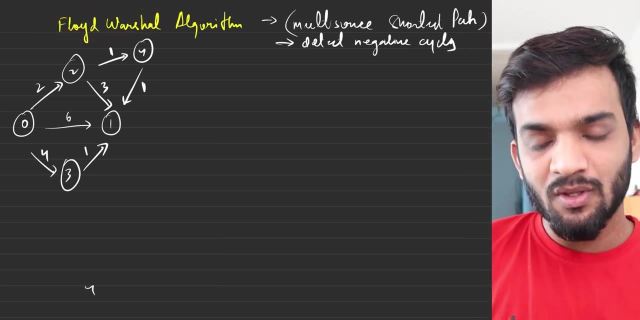 2 to 4. 4 to 1: this is the shortest path. if I'm asking you, that's the definition of shortest path. any path that takes the least amount of edge weights is known as the shortest path. So what is the thought process behind the blurred version algorithm? Now, it's very simple. it states: go. 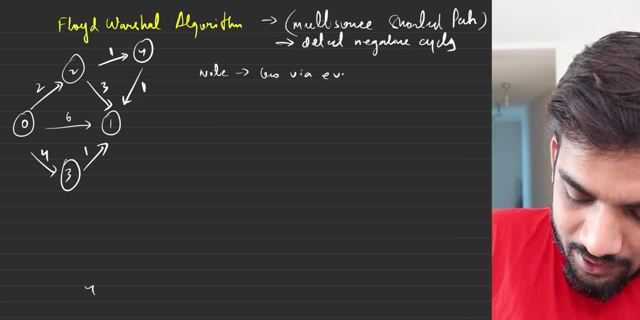 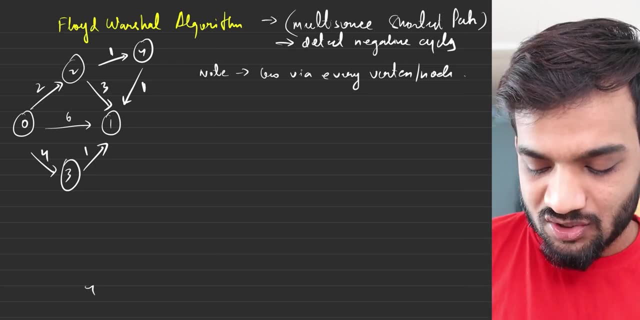 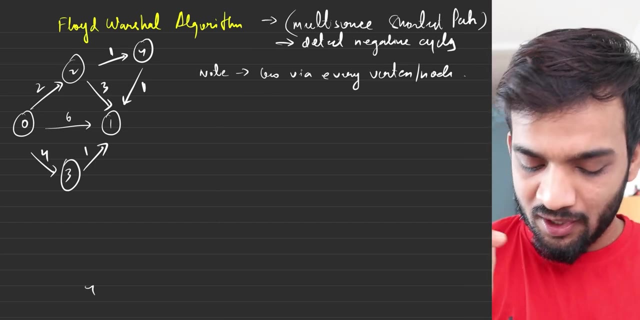 via every edge, go via every node, rather, or go via every vertex or node, whatever you wish to write. so it's very simple. it states: go via every vertex and node, go, go and try, try, try, try and get the shortest one. So for an example, for an example let's take: we want to find from 0 to 1 right. so 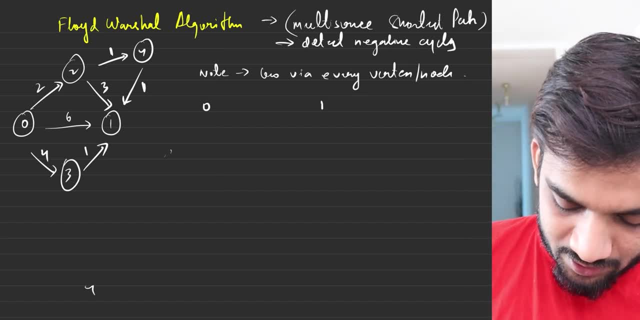 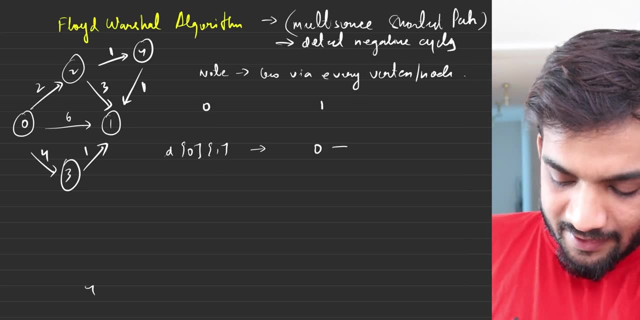 if you're trying to find from 0 to 1. assume the distance you're trying to find is from 0 to 1. okay, what are the possible ways that you can go? you can be like striver: I can go from 0 to 1 directly. 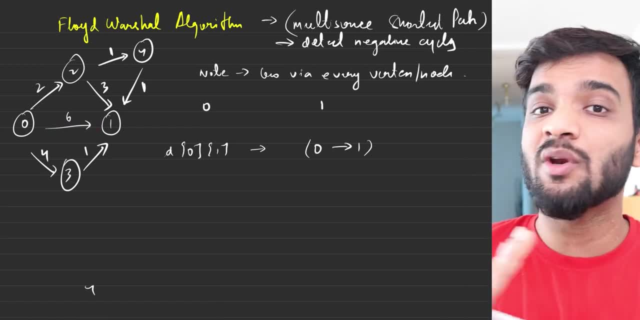 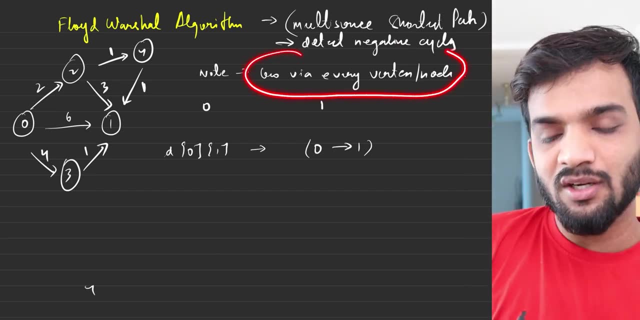 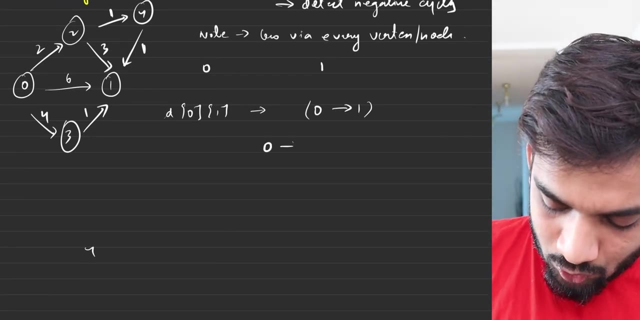 I'll be like, yeah, that does make sense, right, because that's the straightaway path 0 to 1. if there is an edge, I go via that. that's one of the ways. but if I ask you go via every vertex, then you can be like, okay, I can probably go via 2, so which will mean I will go to 2. 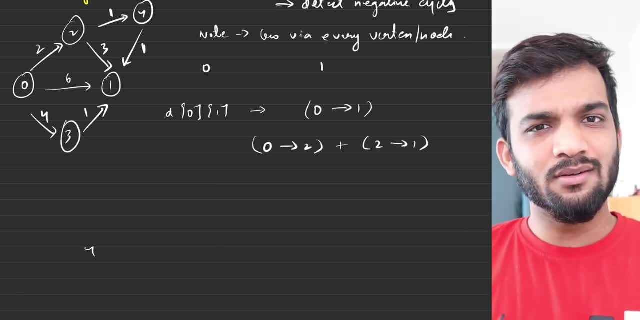 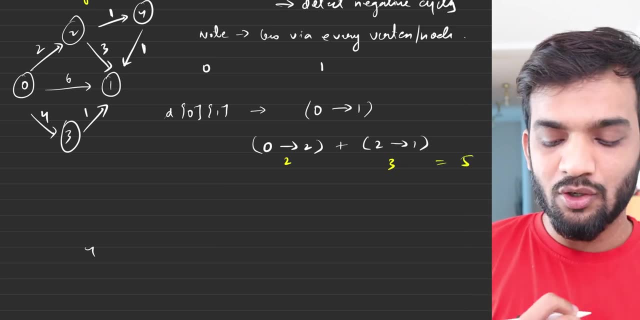 and then from 2 I'll go to 1. does that make sense? yes, and if I go from 0 to 2, it's going to cost me 2, and from 2 to 1 it's going to cost me 3, which will give me a total. 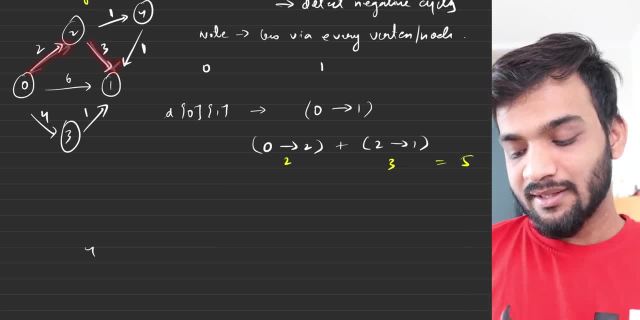 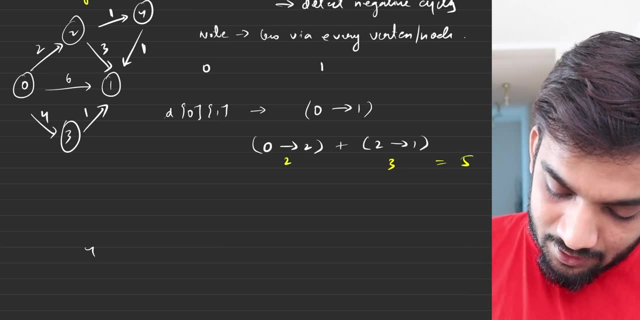 cost of 5, which is nothing but this particular path, that is, if I go via 2. that is, if I go via 2, can I go via 3? I can, so that will be something like: I'll go from 0 to 3 and then I'll go from. 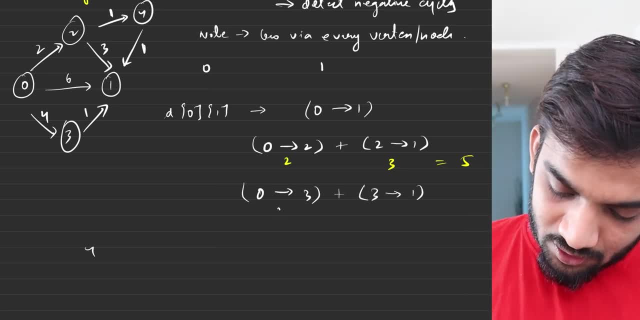 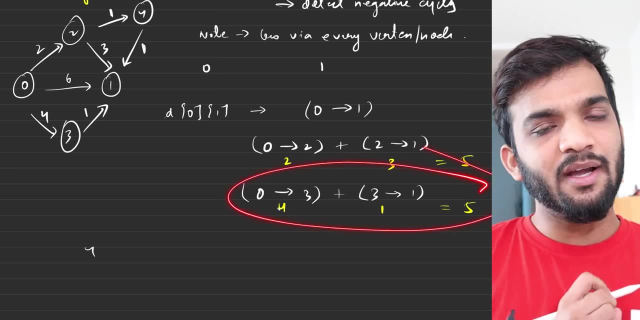 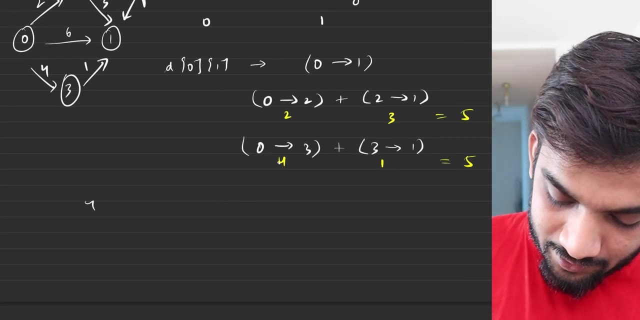 3 to 1, correct. so if I go from 0 to 3, that's going to cost me 4. from 3 to 1, that's going to cost me, which will be a total cost of 5 again. Can I go via 4? I can go via 4. so if I go via 4, let's let me write that in white- if I go via 4, 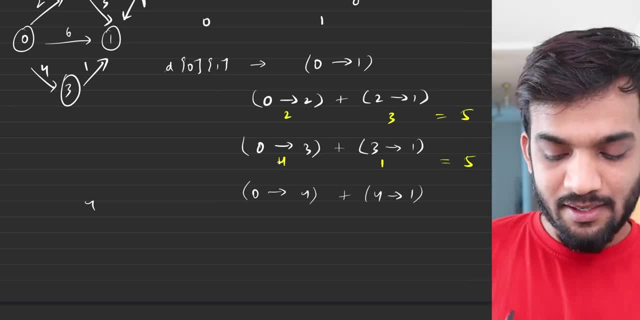 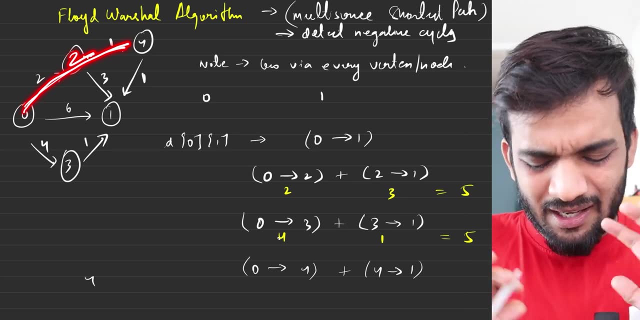 it will be 0 to 4 and 4 to 1 right, but 0 to 4. if you see, it's not direct path, it's a path via 2, probably someone would have computed. assume as of now, someone has computed that and given you. 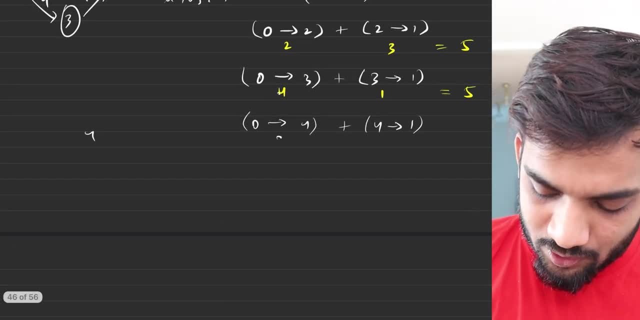 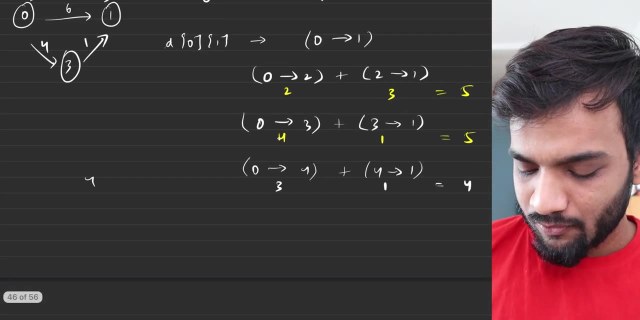 from 0 to 4, it's a 3. okay, so I'll be like: okay, 3, and from 4 to 1 it's a 1, so a total of 4. so apparently we notice that from 0 to 4 and 4 to 1, it's taking me a cost of 4, which is indeed. 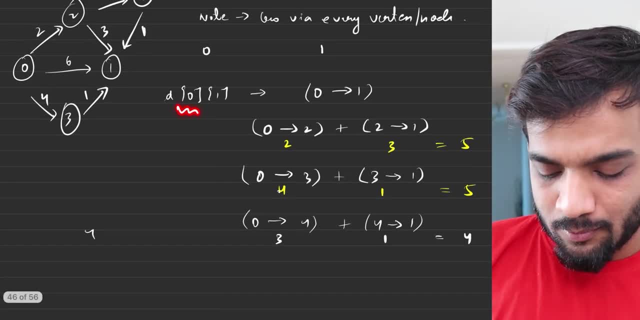 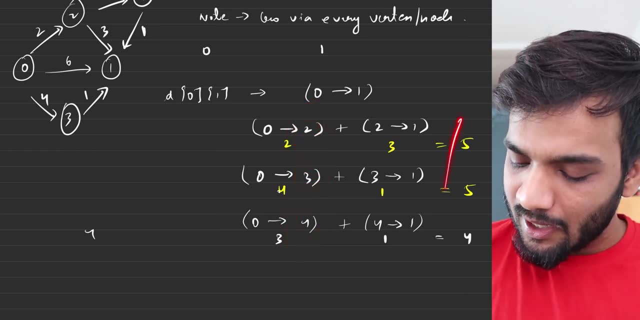 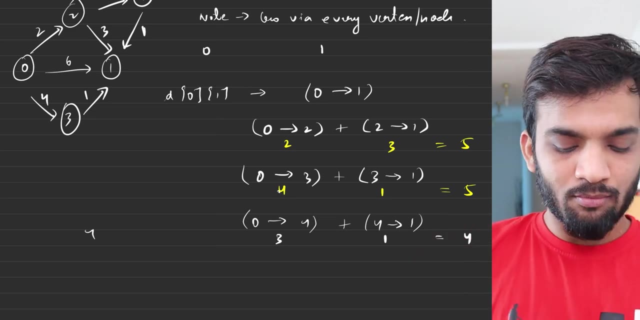 the shortest one. so what I did was, in order to go from 0 to 1, I tried out. every different vertex can be 2, can be 3, can be 4, and apparently I took the minimal path and this is what it is. so the logic is very simple: assume all the vertex are from, like the 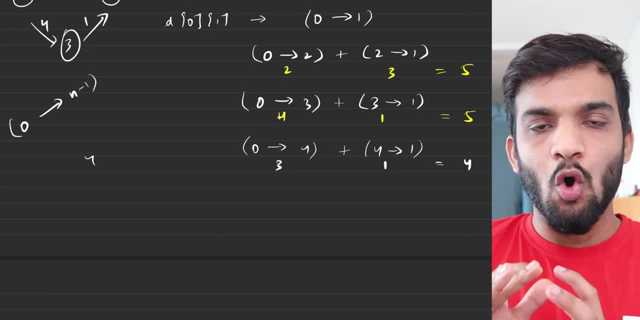 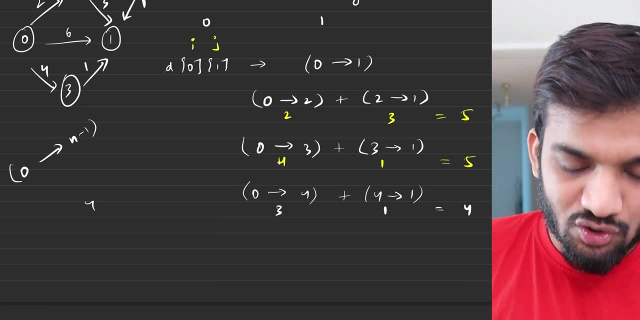 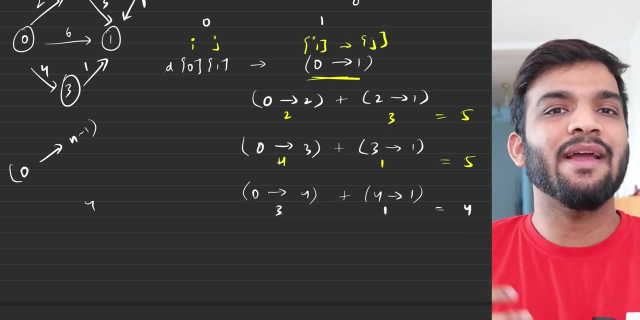 vertexes are definitely from 0 to n minus 1, so I can say all the vertex. so if I'm trying to look, can I say if some, somewhere down the line, if this is i and this is j, and can I say this is nothing, but I go from straight i to j, which is nothing but the edge itself, and can I say this, this, this. 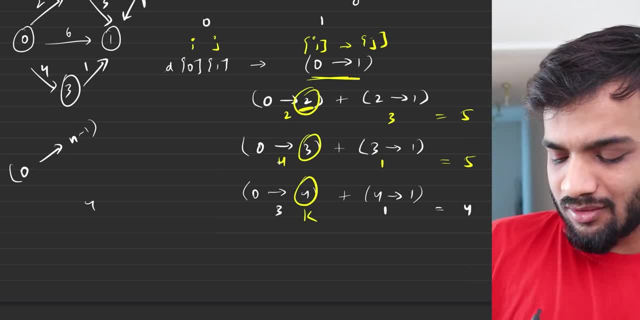 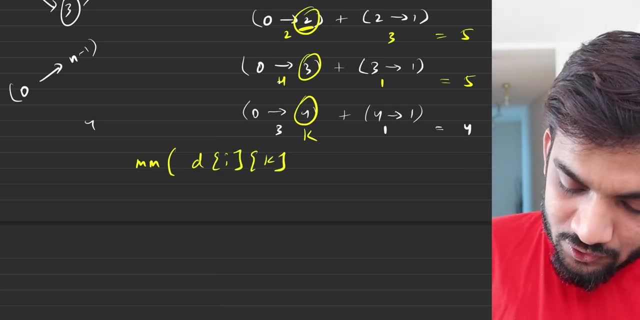 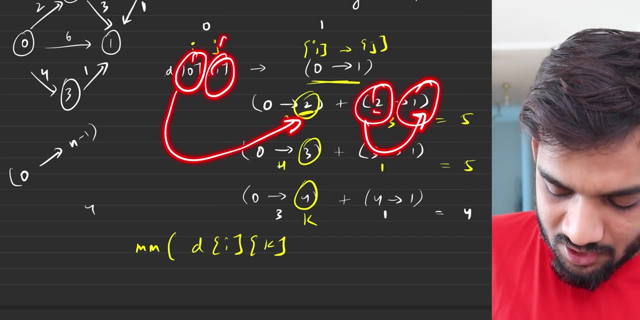 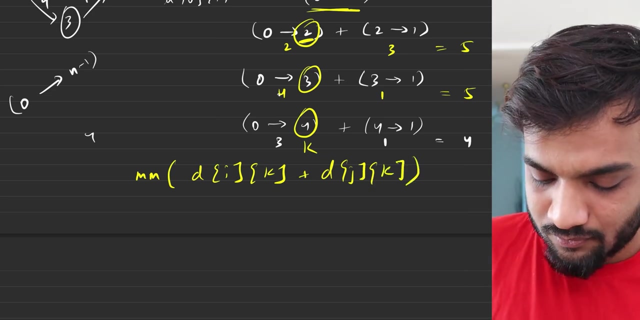 to be k, assume. so can I write the path to be minimum of? if you try out all the k's, it will be from i to k. very obvious, because you go from 0 to 2 and then from 2 to this, which is nothing but the j, correct. so can I write this plus j of k? I can. that's what the path is from i. 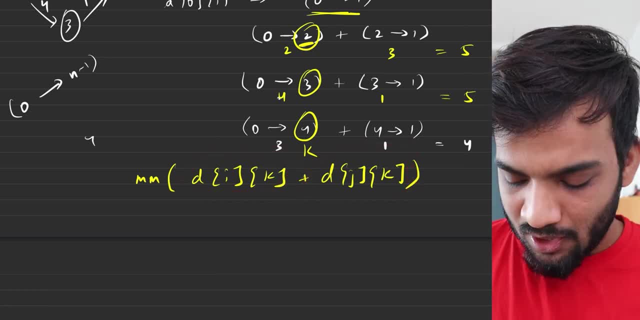 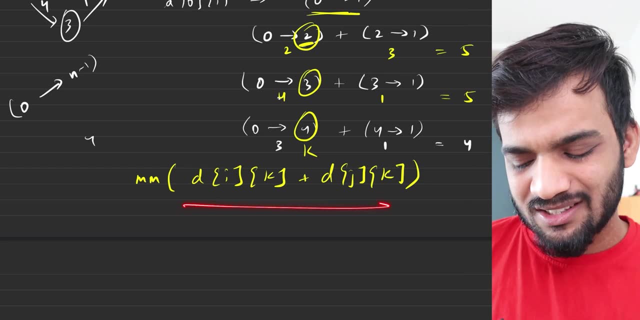 to k, I'll go, and from j to k is what I have to go, and if I take minimum of all of them- 5, 5, 4 minimum- I'll have the answer somewhere down the line. I've understood, but I need to implement this on a wider 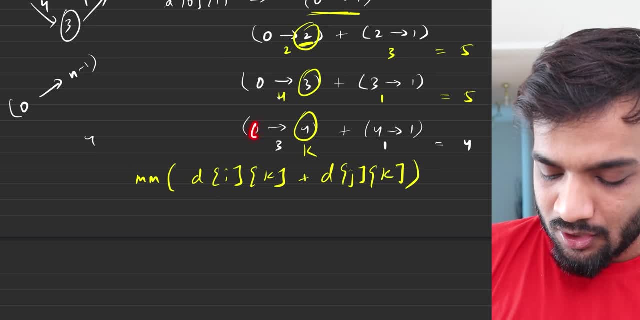 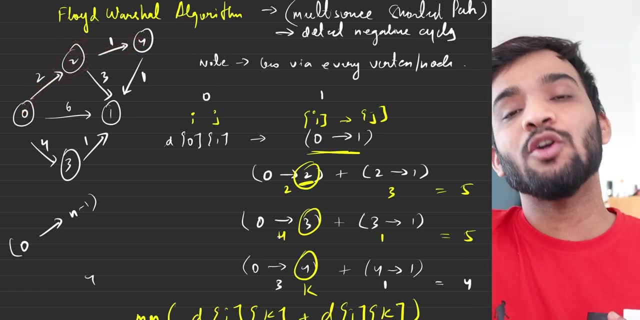 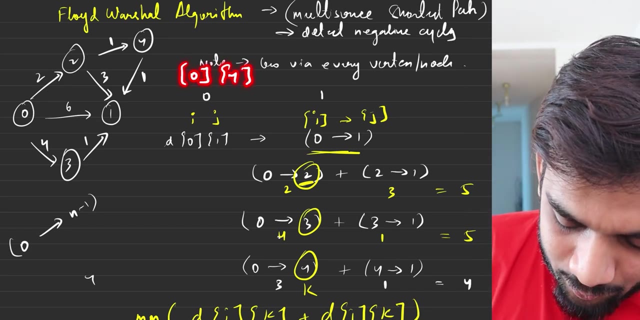 scale. what do I mean by a wider scale? because over here 0 to 4 was not a direct edge, because 0 to 4 meant it went via 2. so it was going via 2. so somewhere down the line in the past, someone would have also computed 0 to 4 and they would have implemented via 2, understand. so 0 to 4 would. 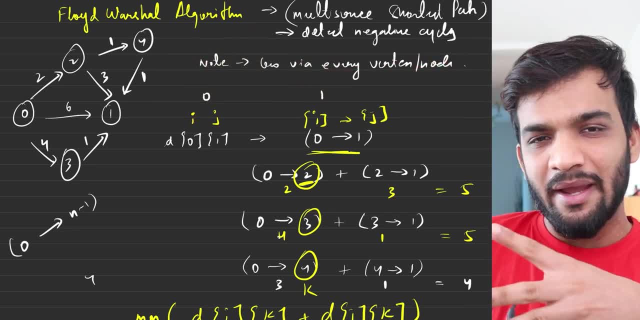 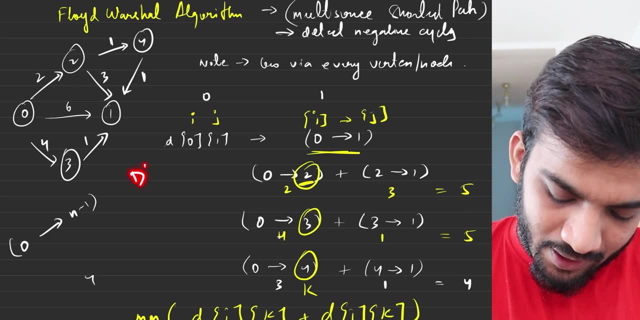 have been computed and stored. so this is where you get an idea: okay, something like a dynamic programming, because we're using something which has already been computed. so you get an idea that, okay, this is a dynamic programming solution. it's not necessarily that you know dynamic programming. 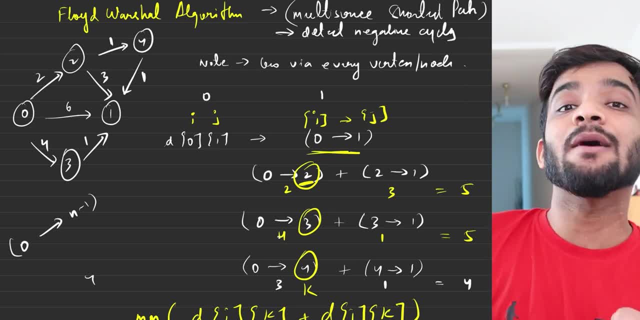 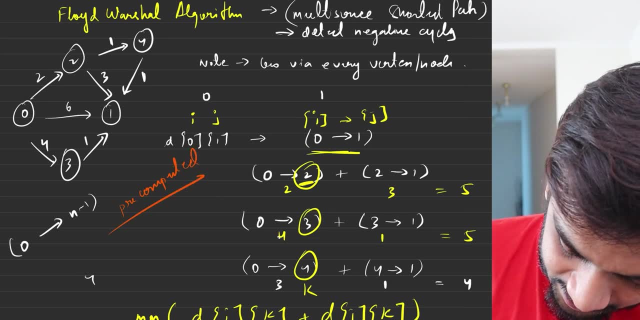 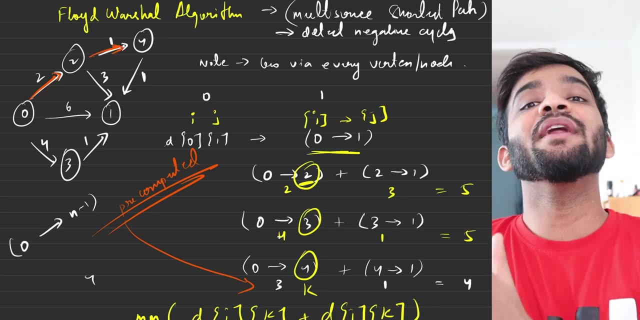 I'm just saying: try to relate. we're using something which is pre-computed. if I write it properly, I can write something which is pre-computed, which was, in this case, this one, because 0 to 4 was pre-computed, you did not compute. at the point, someone already knew what was the value to go. 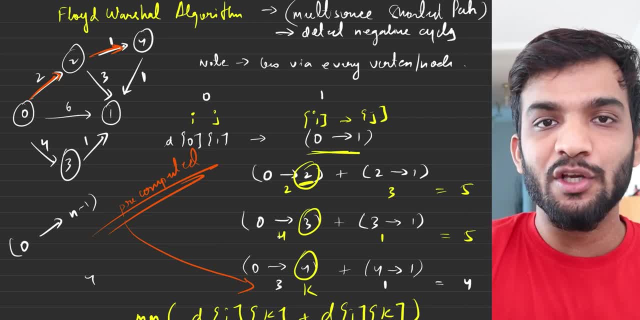 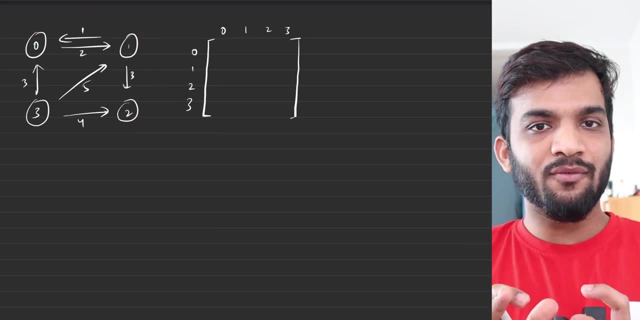 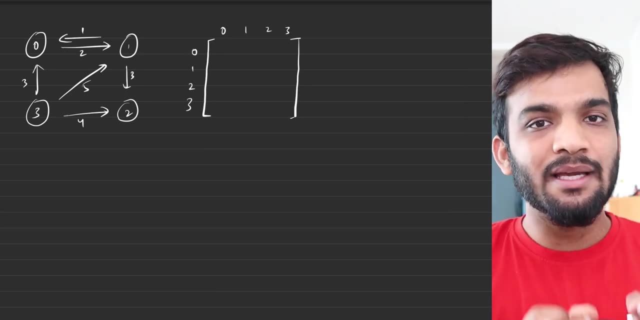 from 0 to 4. that is what you need as a pre-computation. so you pretty much got the formula. now what I'll do is I'll try to give you a sense of the graph and then slowly and slowly, step by step, implement this algorithm so that you understand how is this algorithm implemented till. 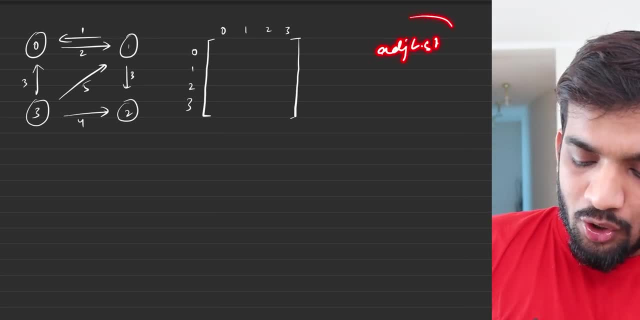 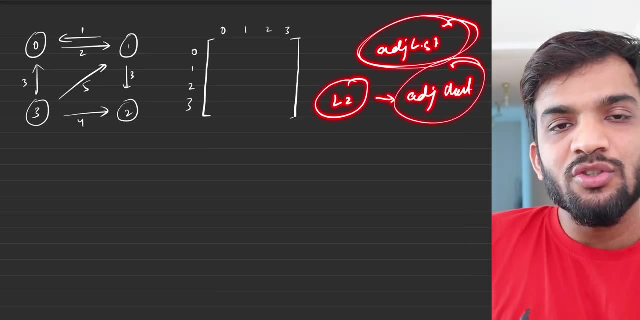 now, in all the problems, we have been using the adjacency list in order to store the graph, but also I've also taught you one more method, which is the adjacency matrix method. so you're going to use the adjacency matrix method in order to store this particular graph. okay, it's very simple in. 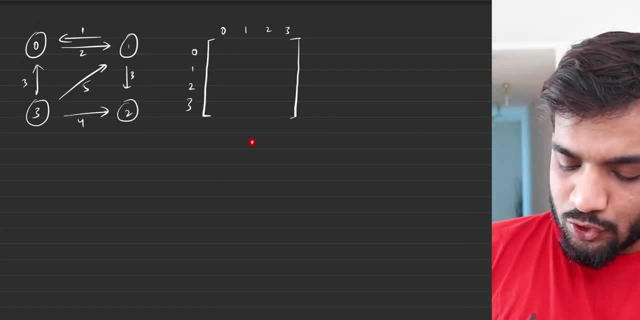 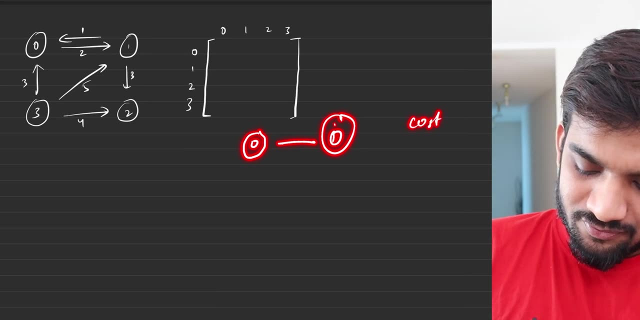 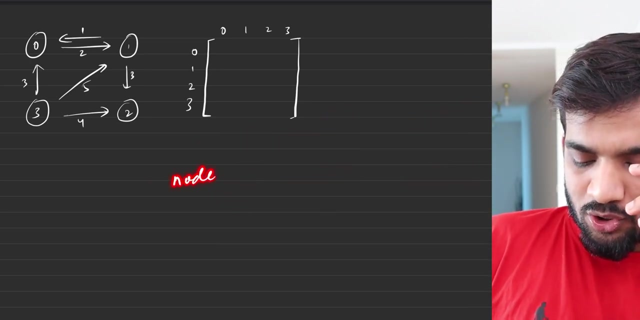 case you haven't seen the lecture too. it's very, very simple. so something we know for sure is: if zero is the node and I want to go to zero itself, the cost will be zero. if I want to go from one to one, the cost will be till zero. so, from any given node to the node itself. 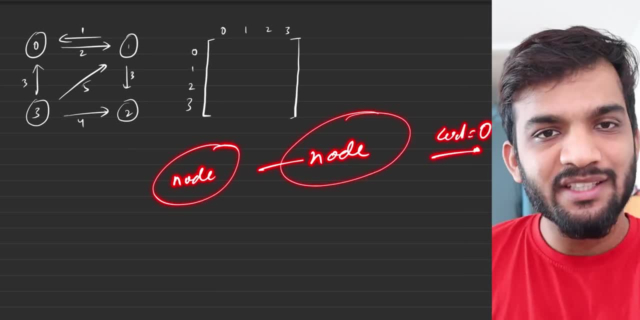 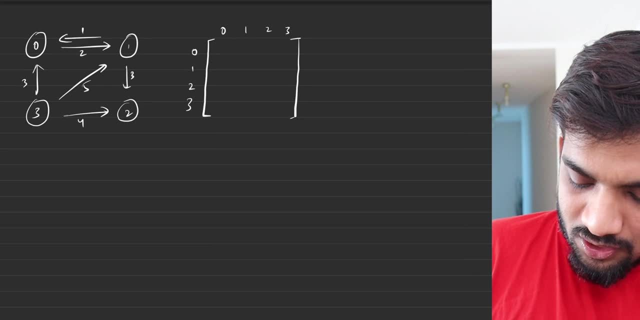 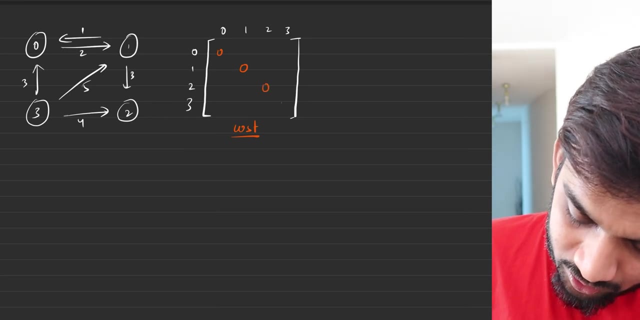 the cost is going to be zero, no matter what you do, because you're already standing in the node, something I know: zero, zero. so this portion will be storing the cost, so I can call this as a cost Matrix. so zero to zero will be zero, one to one will be zero, two to two will be zero, three to three will. 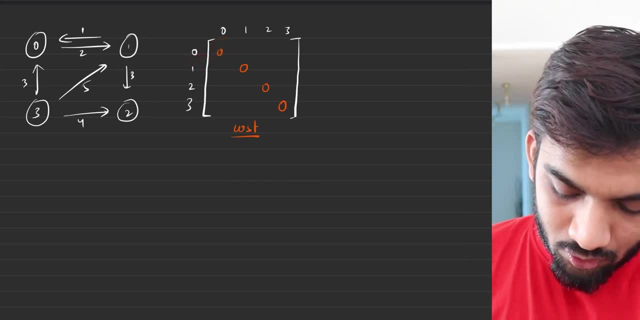 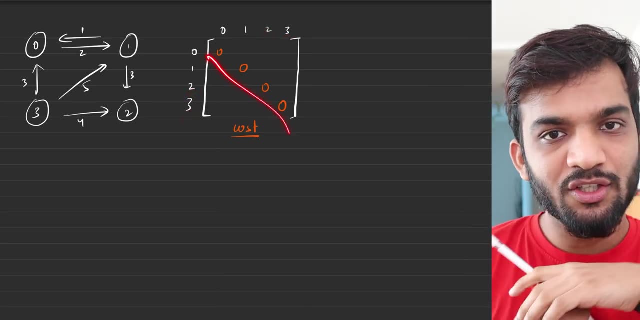 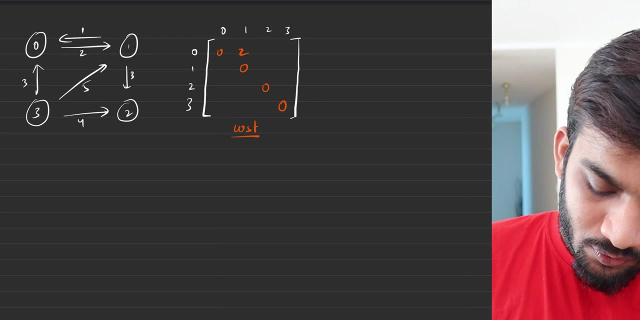 be zero. so basically I'm saying this is zero, zero, zero. this is one, one, zero, this is two, two, zero, this, what are the other? it says zero to one is two, so go to zero, to one and store two. go to zero, go to one and store two. it says one to zero is one, so you go to one, you go to zero and you store one, okay it. 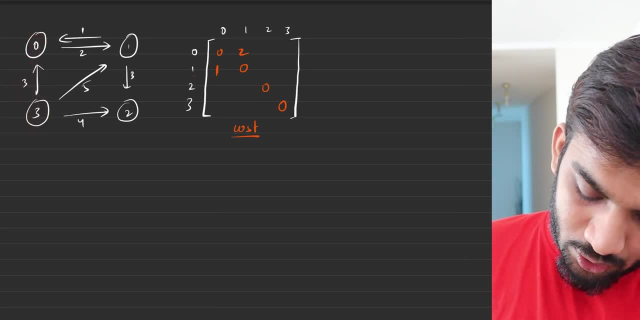 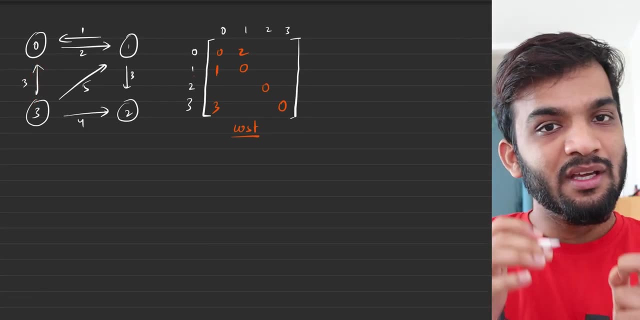 says: three to zero is three. so go to three, go to zero and store three. do not store the opposite vertex, because it's a directed graph. it is a directed graph if it's an undirected graph. for an example, if it's an undirected graph and you want to imply: 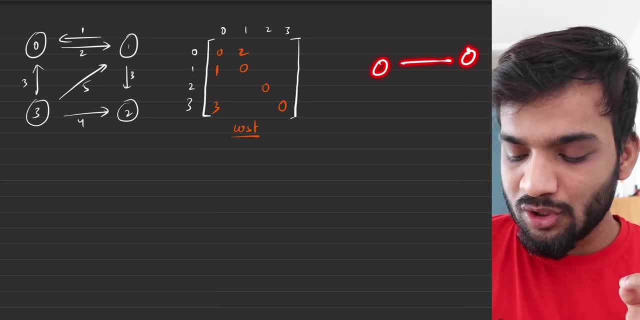 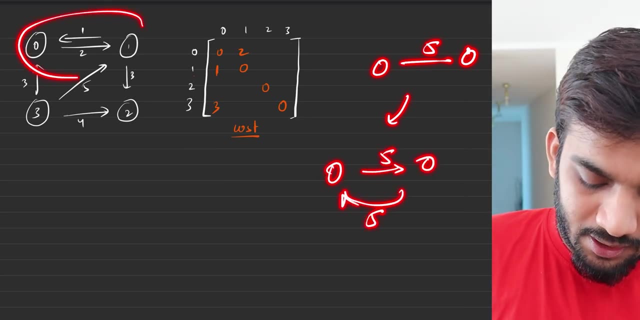 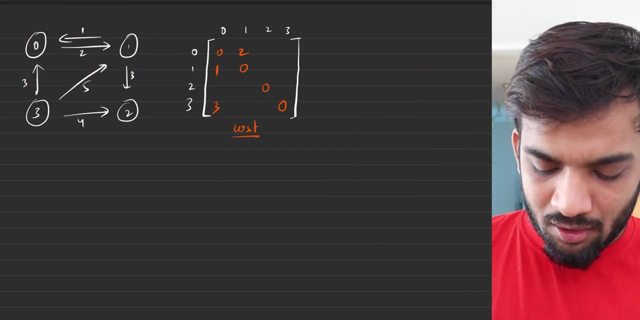 and you want to, uh, apply this Floid version, just split this into something like this: five, five, as you see, our dual Direction Edge, but the different values in undirected. just make sure you assign them same values. now remember you just store three, zero as three, because there is no zero. 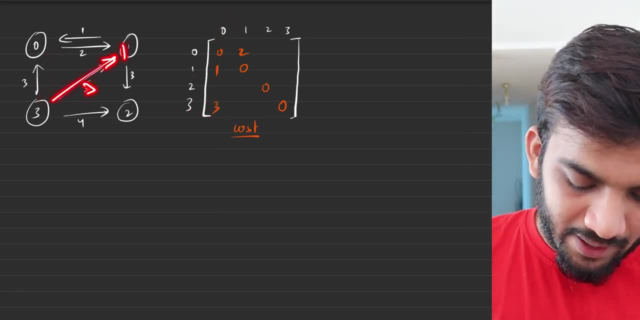 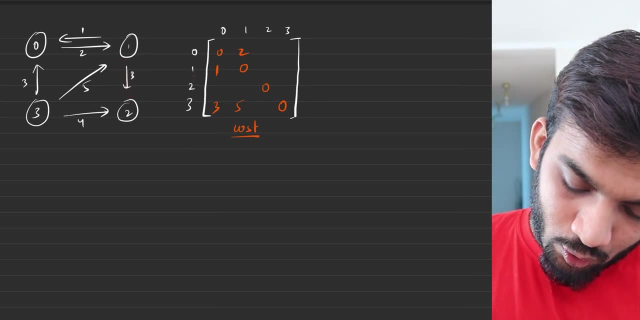 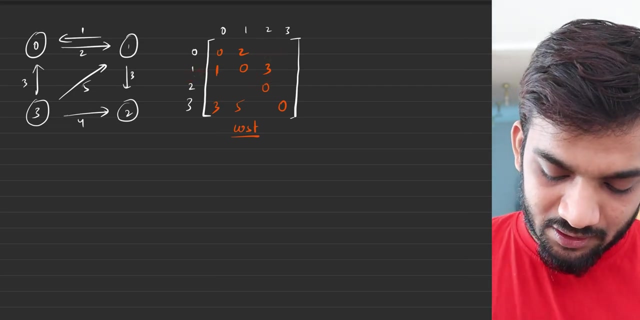 three, okay, nice. next is three. one as five. so go to three and one and assign five. next is one, two as three. go to one and two and assign as three. perfect, one, two, one, two assigned as three. do we have any other thing? one, two, three, four, five. one, two, three, four, five. okay, we have three. 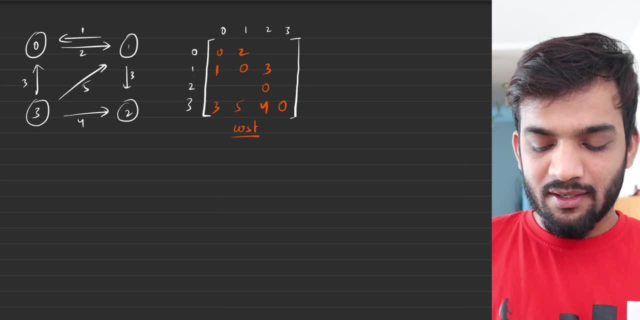 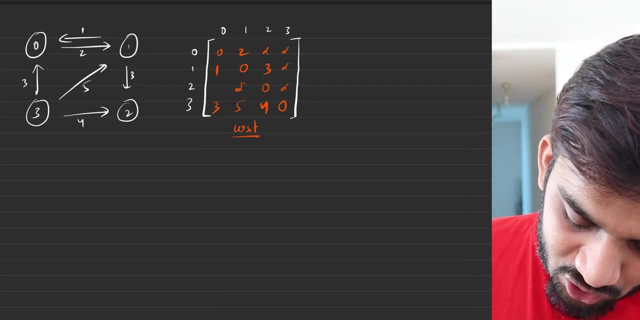 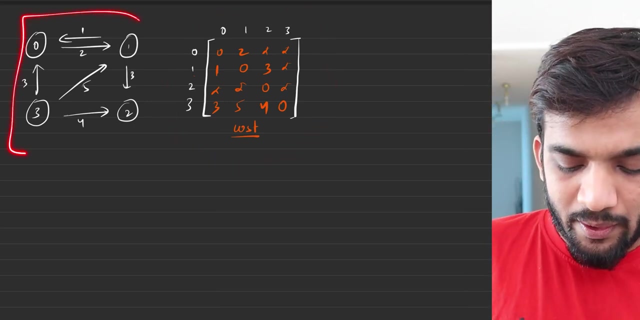 to two as four, three to two as four. done so, what i've done is i've assigned the cost. make sure everyone else is infinity, which means unreachable as of now. which means unreachable as of now. so this is the initial cost matrix, which you can always derive from the given graph. now you must. 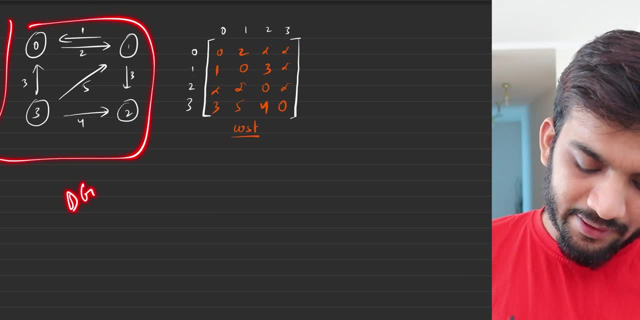 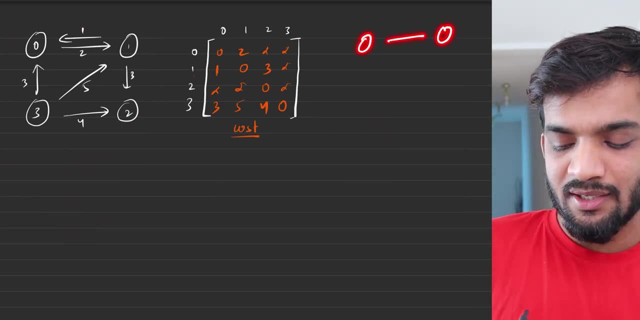 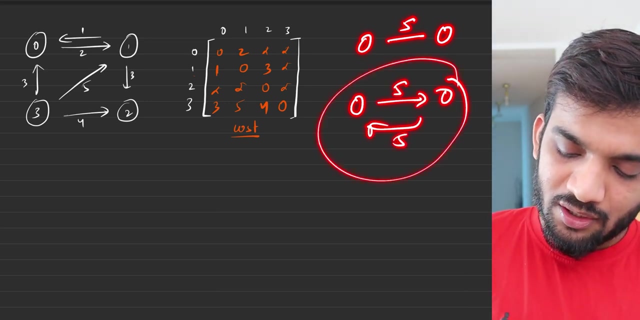 be thinking: but striver. this is a dg, a directed graph. what if it's a ug? how will we implement the floyd motion? very simple: if there is an edge like this and it has a cost of five, you say okay, five this way, five this way. so this is how you convert a ug to a dg: make dual direction edge. 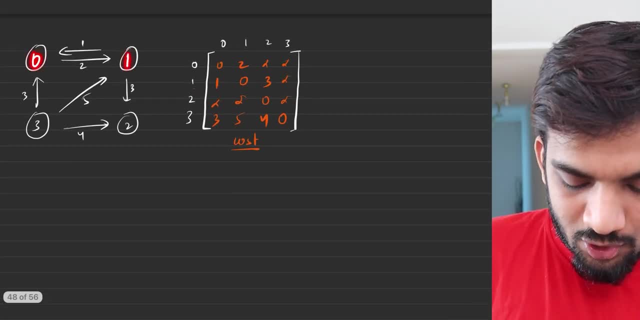 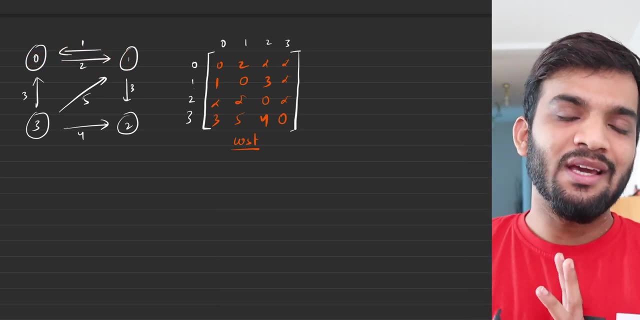 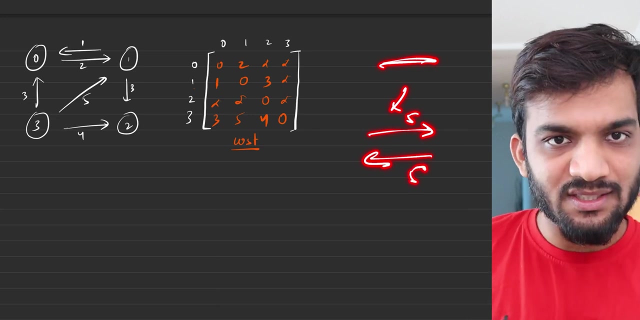 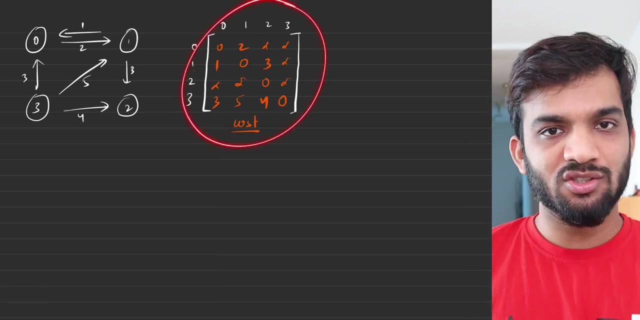 similar to something like this. you see over here there's a dual direction edge, but with different weights. okay, so if you have to apply floyd motion in an undirected graph, just split that edge into two edges of same weights. that's how you can easily convert a ug to a directed graph. so this is the initial cost. 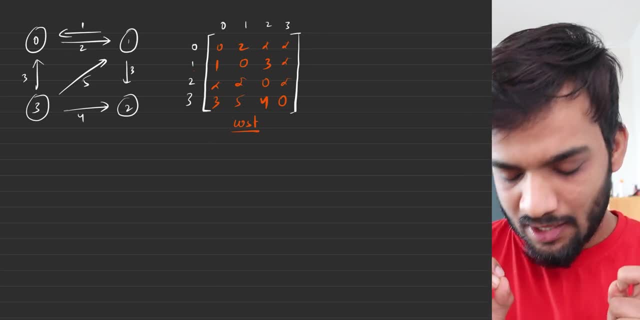 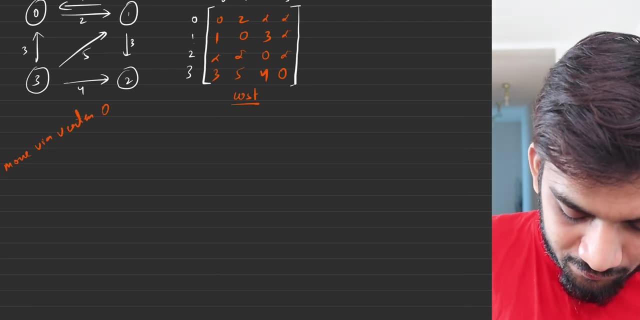 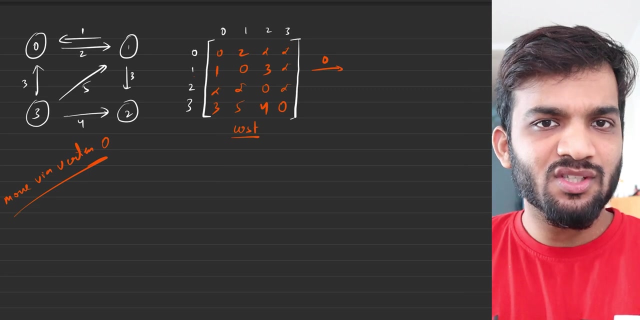 now, what did i say? let's, as of now, assume that i'm going to move via vertex zero. that's my first thing. i'll move via vertex zero. so if i move a vertex zero, i will have some upgraded distance, something for sure. so let's start off with vertex zero and see what will be. 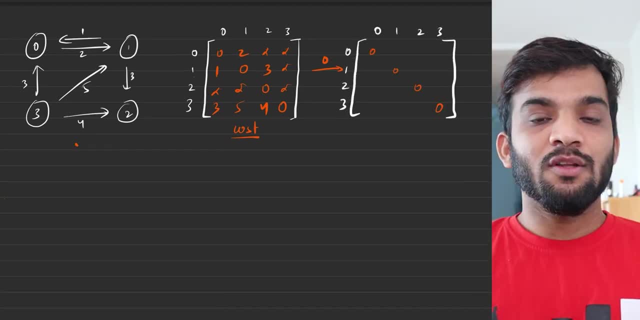 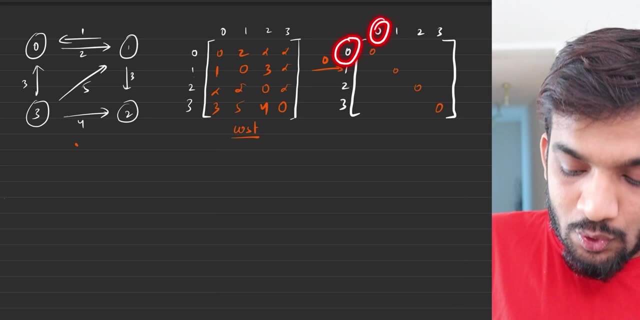 the resultant matrix that we will get. now what i am saying. you have to move via the root zero. so can i say at first, this is zero to zero, stored as zero, next is zero to one, so which means you'll have to do the same thing over and over. so let's say at first, this is zero to zero, next is zero to. 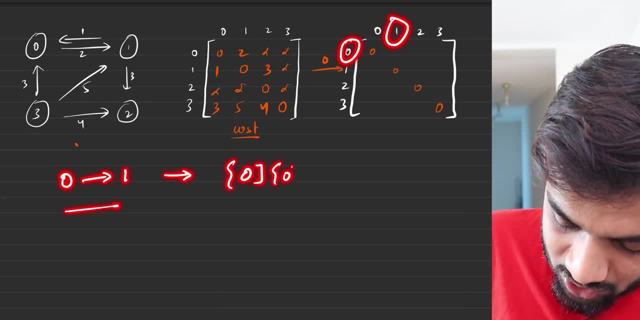 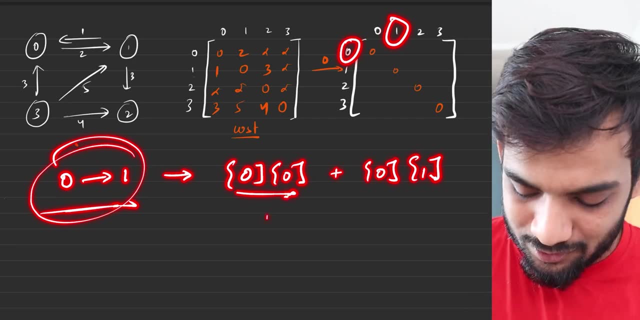 you're moving via root 0, which is 0 to 0 plus 0 to 1. can i say it's similar to saying 0 to 1, because 0 to 0 will always be 0 and 0 to 1 is what we have already stored. 2, so you can just copy paste 2. 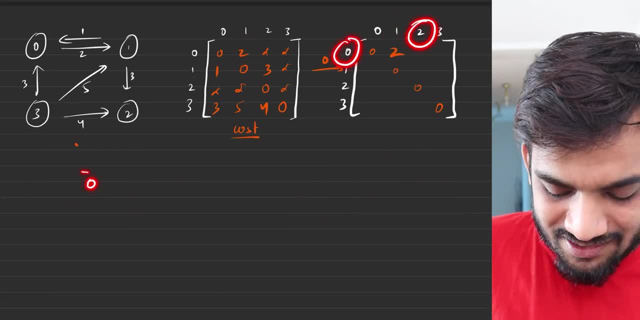 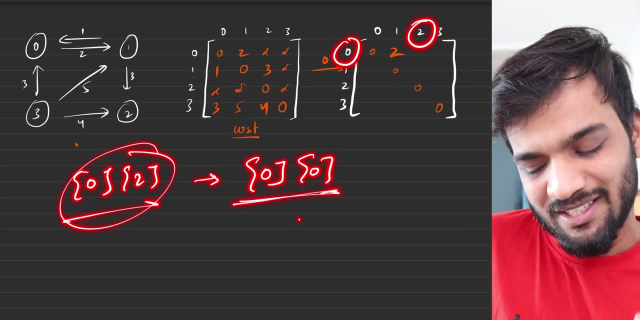 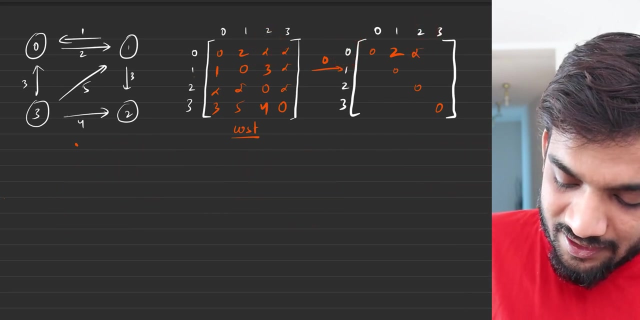 next is 0 to 2. can i say it's similar. 0 to 2 is nothing but saying 0 to via 0. by the way, via 0 means 0 to 0, which is again 0, plus 0 to 2, which is nothing but infinity. so, similarly, this will. 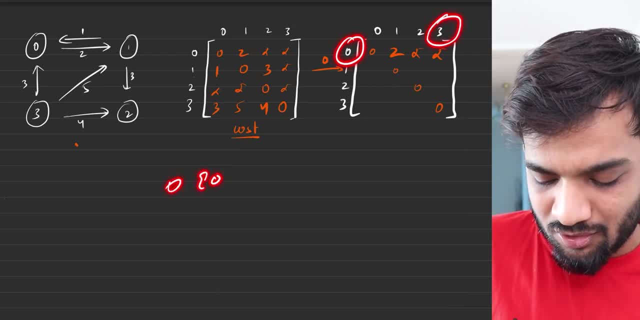 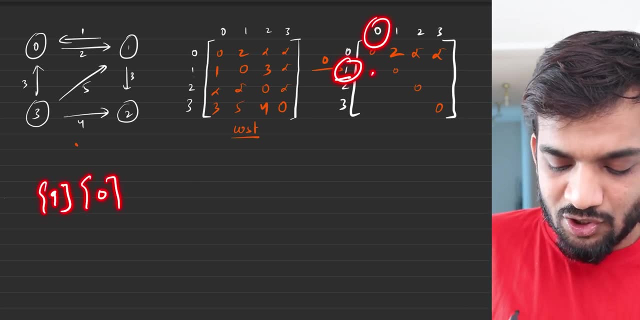 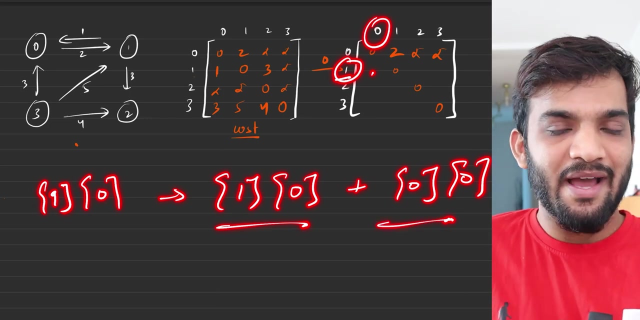 also be infinity. y 0 to 3 will mean 0 to 0 and 0 to 3 similarly, this will mean 1 to 0. what does 1 to 0 mean? 1 to 0 means via, 0 means 1 to 0 itself, and then 0 to 0 via 0 means that only right via. 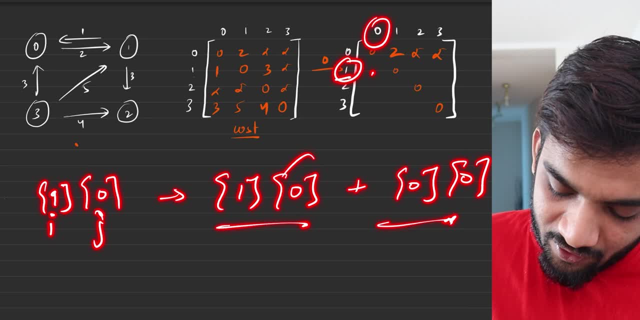 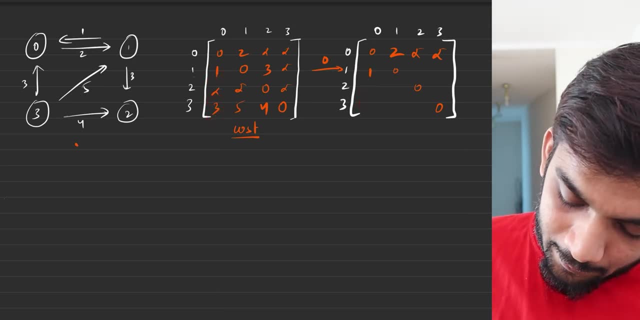 0 means that, because this is i, this is j, you're moving via 0. so can i say: this one, this one, this one will just copy paste these values, just go across. copy paste these values. why? because very simple: if your destination is 0, you can't move via 0, so whatever, 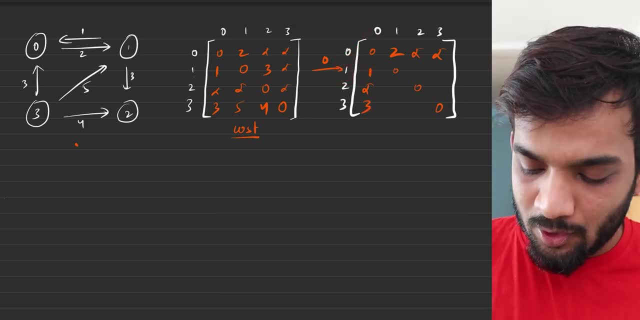 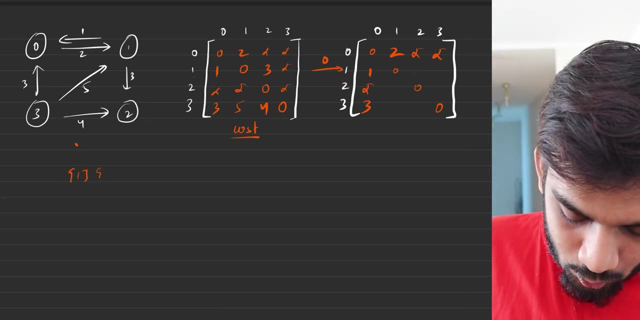 you're taking in order to reach 0. that is what you copy. but what about these places? let's fill them up. so i'm saying: this place is 1 to 2, so i'm saying 1 to 2 via 0, which means 1 to 0 plus. 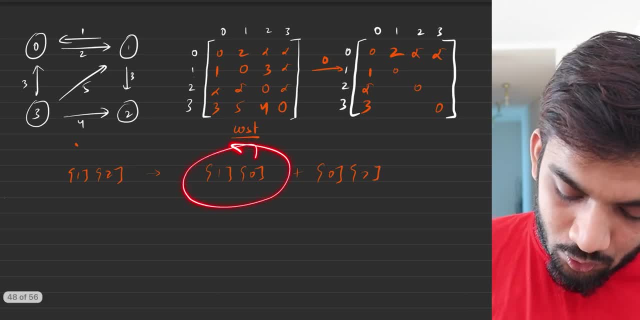 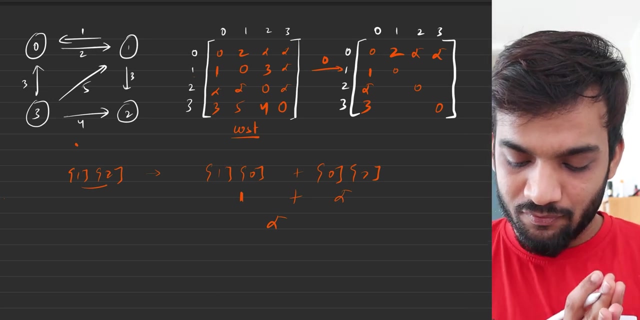 0 to 2. let's see the value of 1 to 0. 1 to 0 is 1, so i'll just write 1 plus 0 to 2 plus 0 to 2 is infinity. so that means it's an infinity which i do not need to write. so what i'll do is: i will keep it as of. 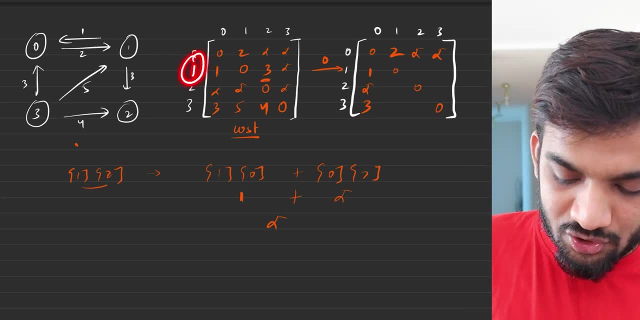 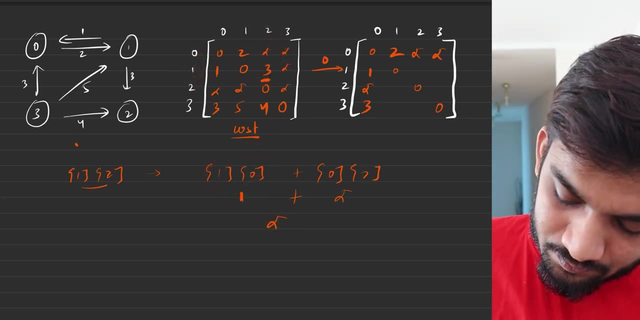 now, and whatever is the value, because i know, in order to reach 1 to 2, i'm taking 3, and if i go via 0, i'm taking infinity. so 3 is a better option. so let's keep 3. no offense, let's keep 3. next one: 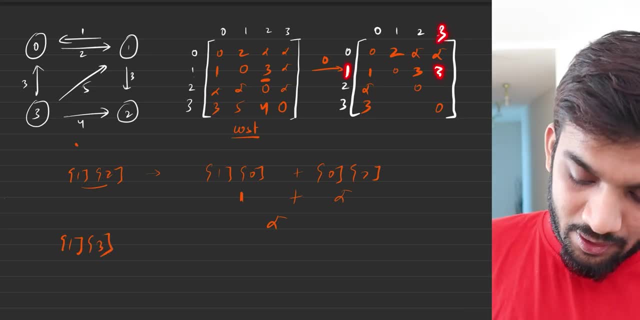 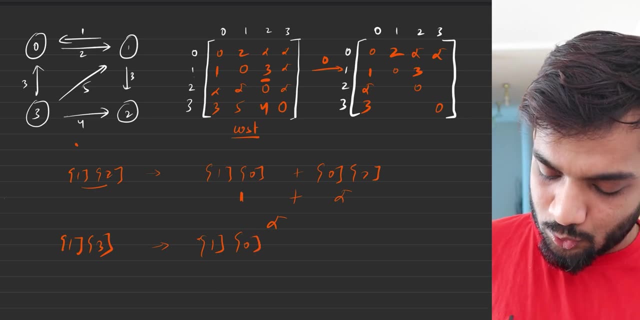 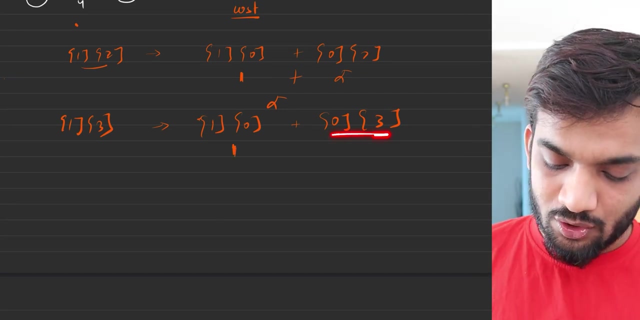 1 to 3. you see, next one is 1 to 3. okay, so for 1 to 3 it will be. i'll go from 1, sorry, i'll go from 1 to 0 plus 0 to 3. now, what is 1 to 0? that's 1. let's see if. what is 0 to 3? so 0 to 3 is again. 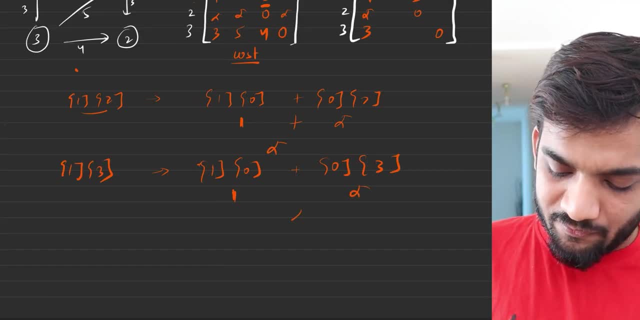 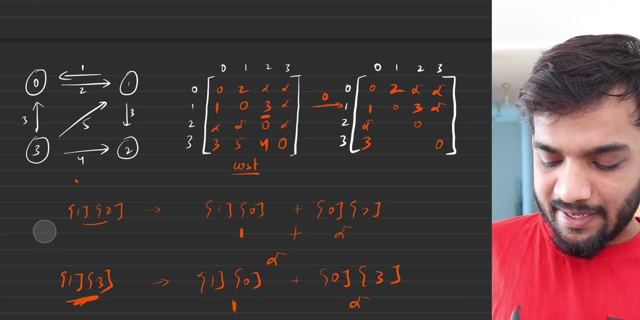 infinity. so if you go via 0, you'll again get infinity. and for 1 to 3, are we reachable in 1 to 3? no infinity, we'll just copy paste infinity. so similarly, if you go via 0, you'll again get infinity. so, similarly, i can say: this is done. similarly, what i'll do is i'll figure out the. 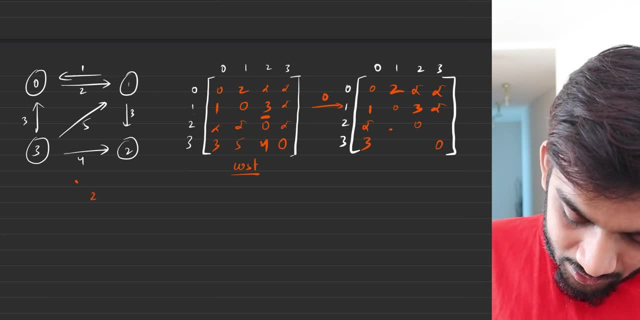 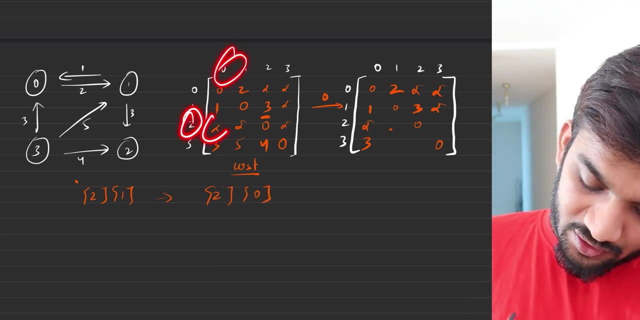 next guys, which is this, which is nothing but 2 to 1. now, 2 to 1 via 0. let's see. i'll go from 2 to 0. how much is it? 2 to 0 is infinity, so the path will not be considered. next, i'll do 2 to 2. so if i go, 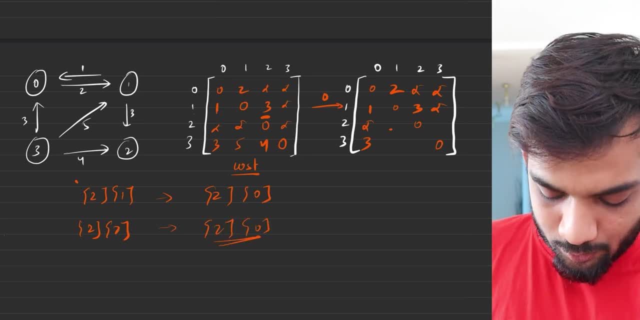 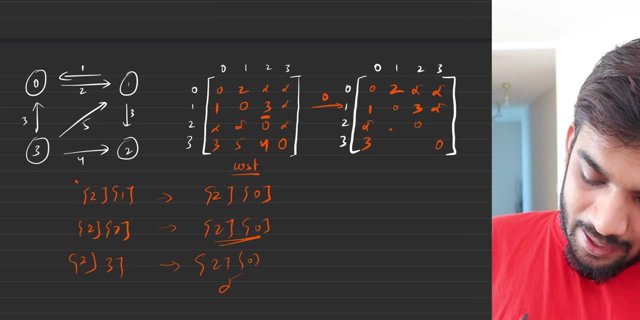 again 2 to 0: it is again infinity not to be considered. next i'll go 2 to 3, which will be via 0, which is again infinity not to be considered. so apparently everyone else is infinity in this case because it was previously infinity. 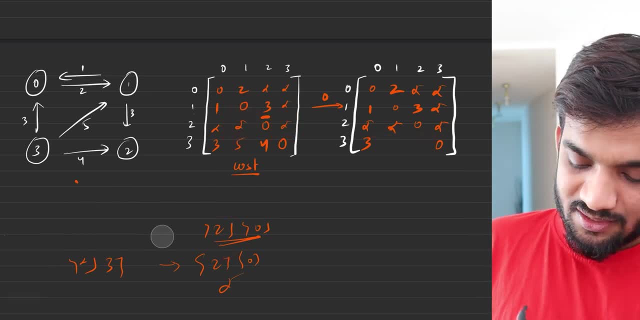 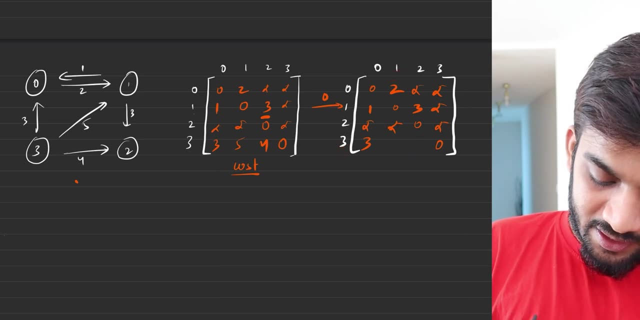 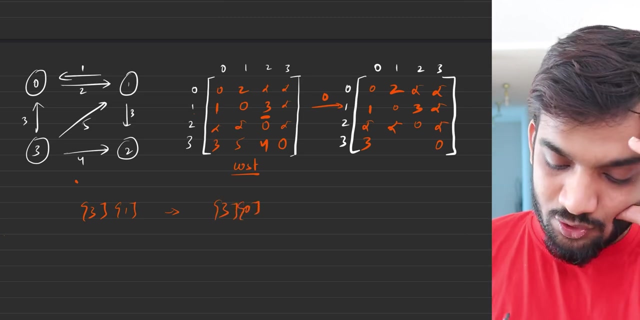 now also, i'm getting infinity, so infinity, infinity, proper. next, let's take the next part, which is somewhere: this one, this one and this one. okay, so 3 to 1. let's see if we can get something better. 3 to 1, what am i saying? via 0, via 0, let's see if i go via 0, which is 3, 0, 3, 0 is 3. okay, 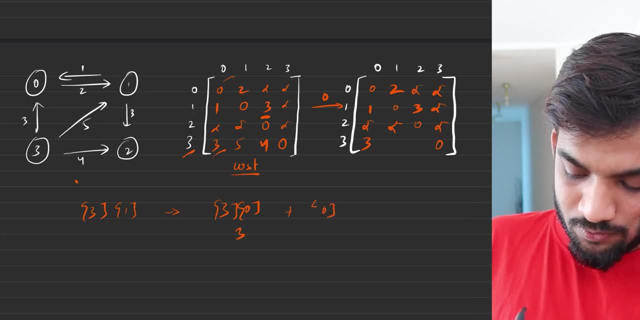 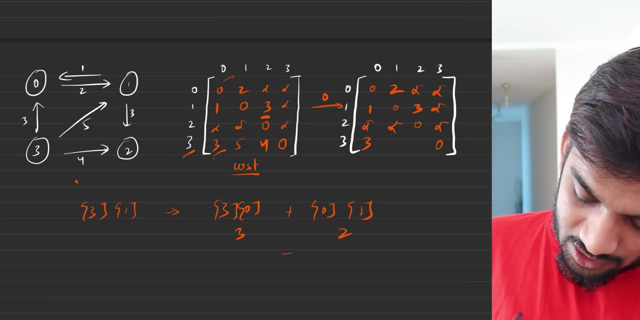 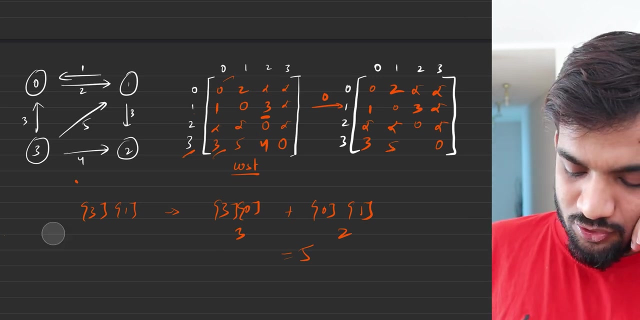 perfect, plus 0 to 1, because i have to reach 1. so 0 to 1, 0 to 1 is 2, so that gives me a total of 5, which is already what i'm taking. so nothing better. we just copy paste the values. we just copy paste the values. 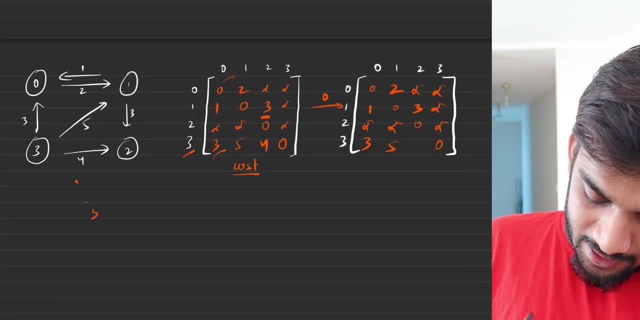 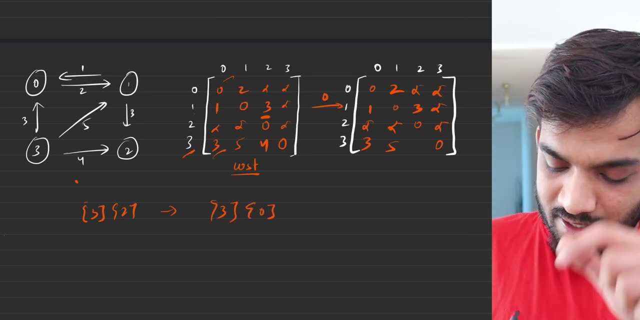 so 3 to 1 is done. let's get the next guy. what is the next guy? i'm saying 3 to 2, which means i'll go via 0, which is 3, 0, right, plus 0, 2. let's see what's the value of 3: 0. 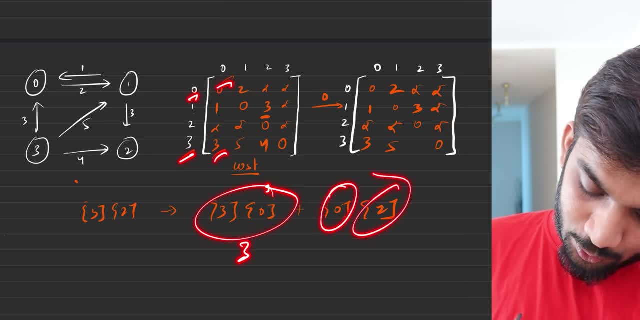 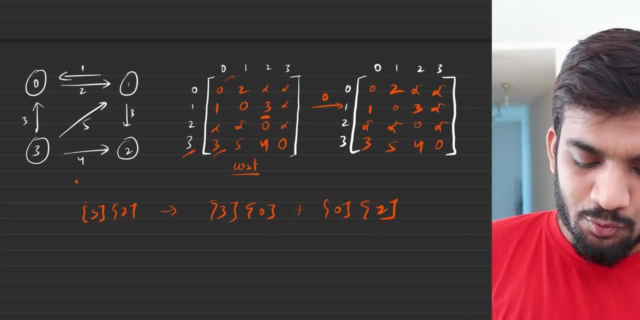 3, 0 is 3. what's the value of 0, 2, 0, 2 is infinity, nothing better. so you're already reaching 3, 2 at 4. we'll keep 4, perfect. so this is what happens if i try to go via 0. so via 0, via 0. i built all the. 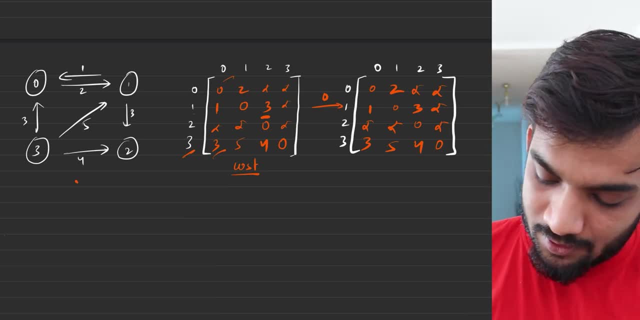 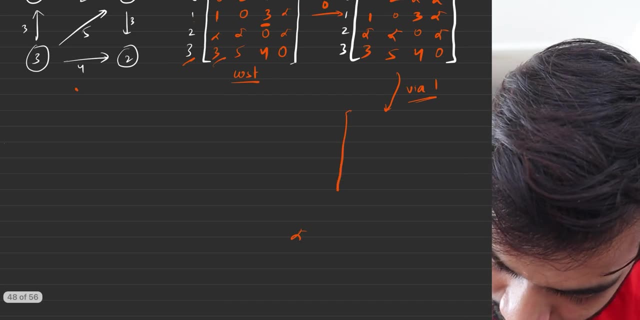 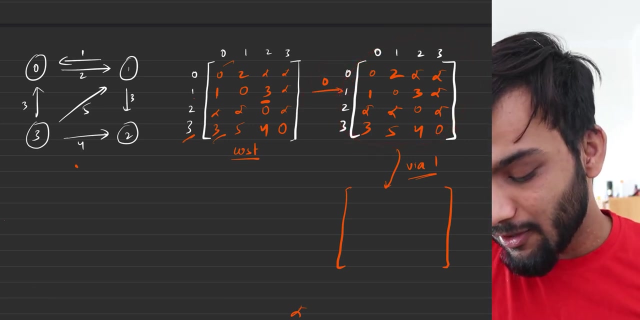 paths. all the paths have been built. let's move to the next one. so next one, i'll say via 1. let's go via 1 and see what is the new, because, remember, via 0 path has been built here. via 0 path has been built here. i'll figure out the via 1 path now. 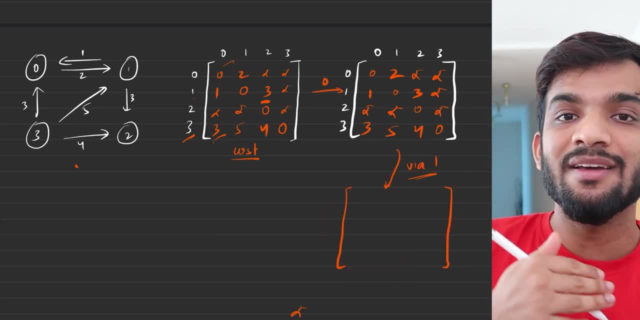 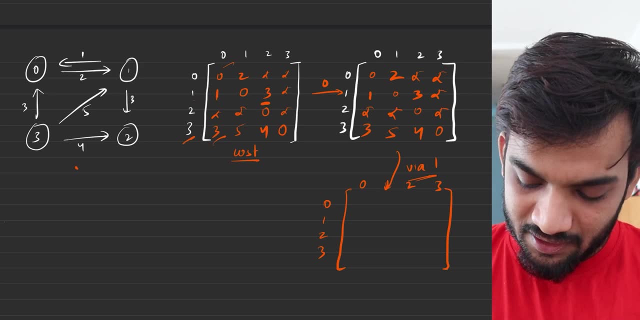 once i figured out the via 1, i'll figure it out via 2, via 3 and so on. we'll get all the answers. so, again, we know if, even if i go via 1- something i know for sure is- these guys will be 0. 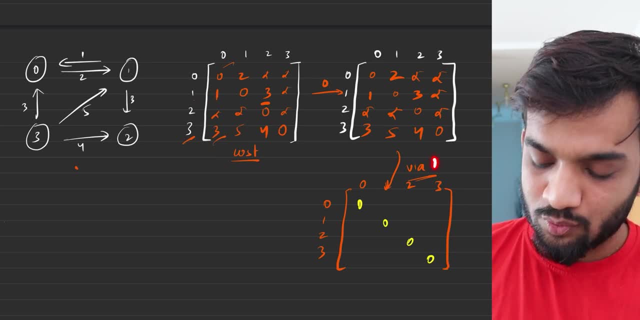 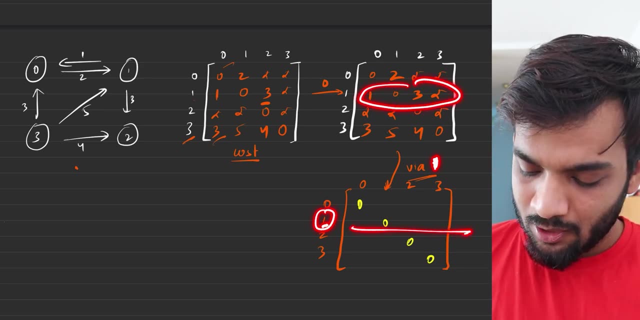 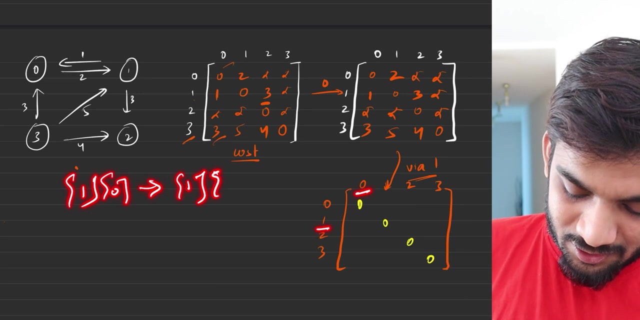 note to note, and anyone who goes 1 like, if the source is 1 like, for this guy this entire portion will be nothing but this. why? because if you're trying to reach 1- 0, it actually means 1 to via. 1 means 1 to 1. 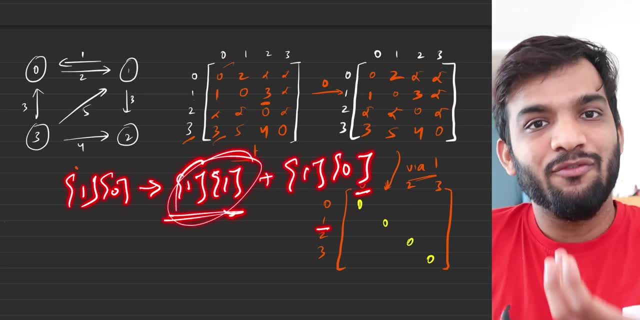 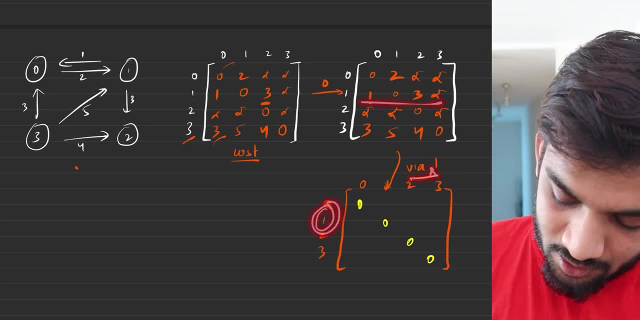 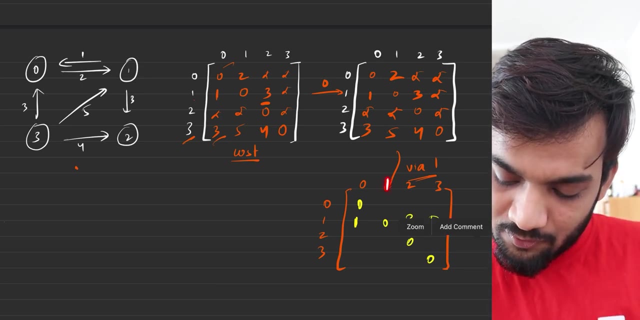 plus 1 to 0. so you're actually going to himself. only if you're saying starting from 1, going via 1, it doesn't make sense, so you just copy paste whatever is there. you just copy paste 1, 0, 3 and infinity. similarly can i say: if this is 1, the destination, it still doesn't make sense via. 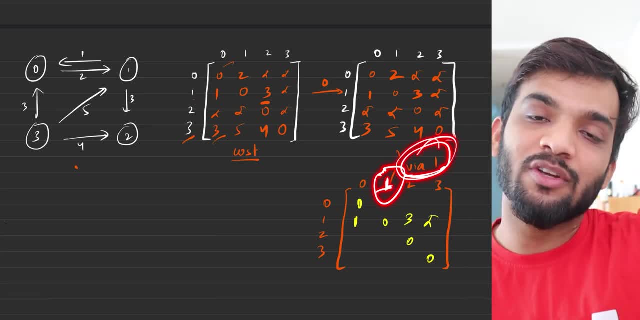 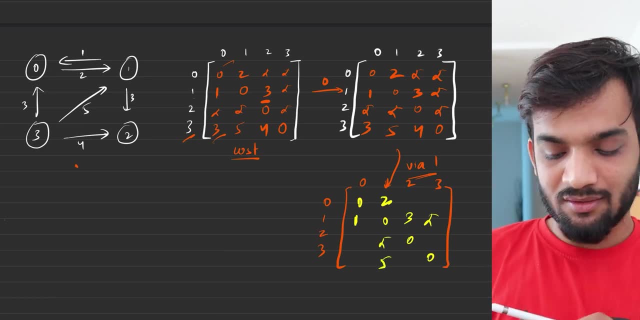 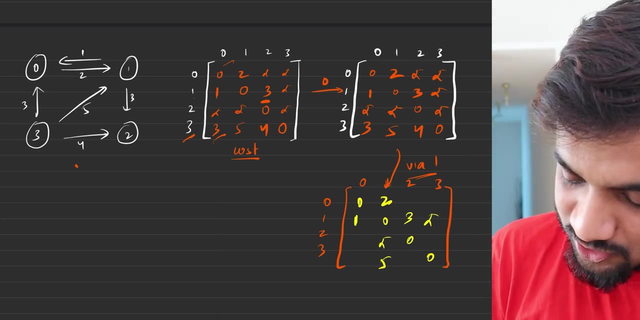 1 and reaching 1. will that make sense? going via 1 and reaching 1? well, that makes sense. no, do you copy paste this row as well? 2, 0, infinity 5: done, copy paste it. so now let's compute this, this, this, this and this, this: five values left are to be computed. let's do it so. first one is 0. 2 via 1. 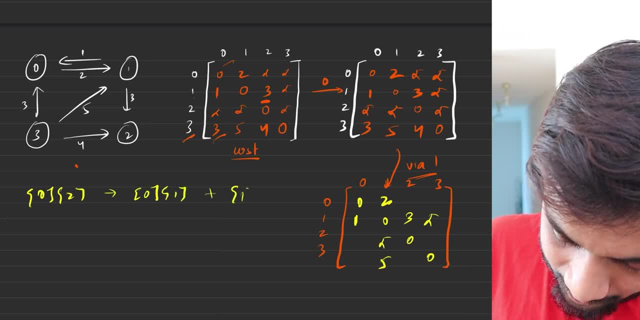 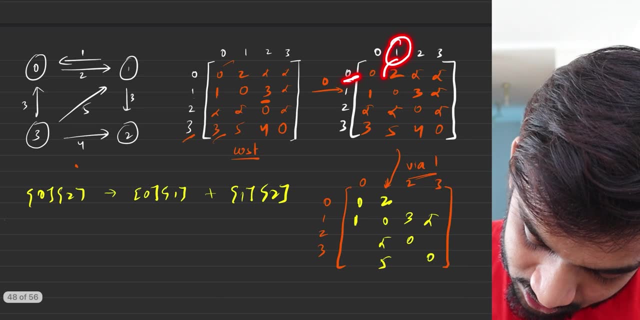 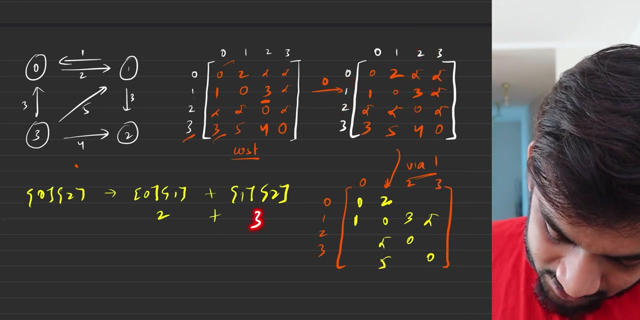 means 0, 1 plus 1, 2. let's compute this. so 0, 1 means 0. sorry, you will take this 0 and this one, which is 2, so 0, 1 means 2 plus 1, 2, 1, 2 means 3, you get a 3, which makes it 5. what is? 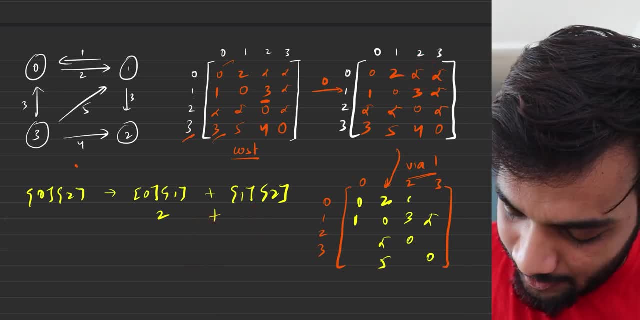 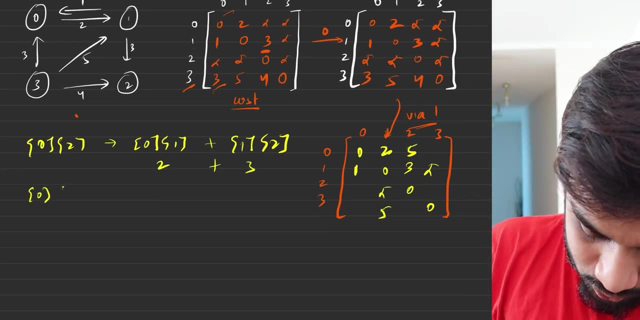 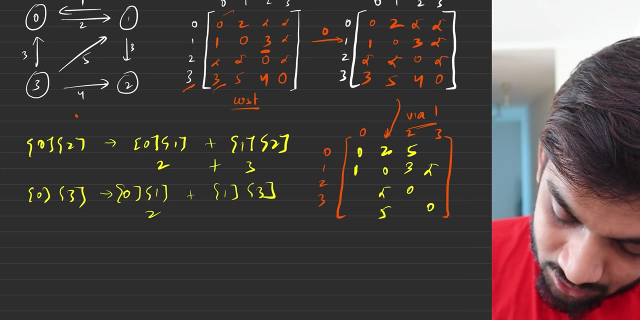 the value already stored: infinity. you are reaching at a better position- 5. you go via 1, you're reaching at 5. much better, much better. next, 0. 3 via 1 means 0. 1 is 2 plus 1- 3. let's see the value of 1- 3. so if 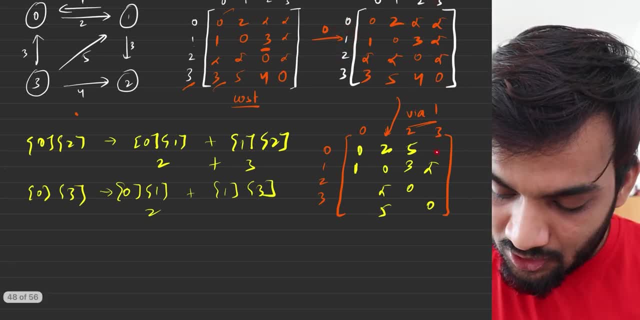 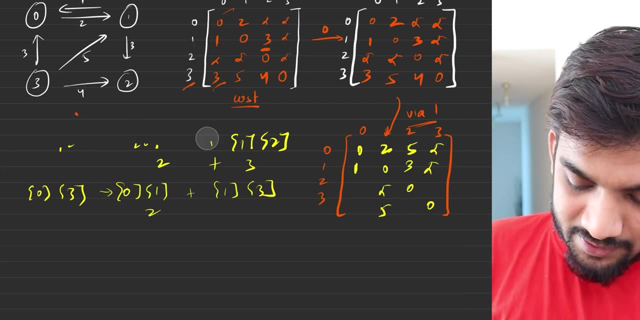 i take the value of 1 and 3- that's infinity- not to be considered. so whatever is the value, we'll just copy paste: perfect, let's copy paste the value: amazing. next, let's erase this. let's go to the next row. if i go to the next row. 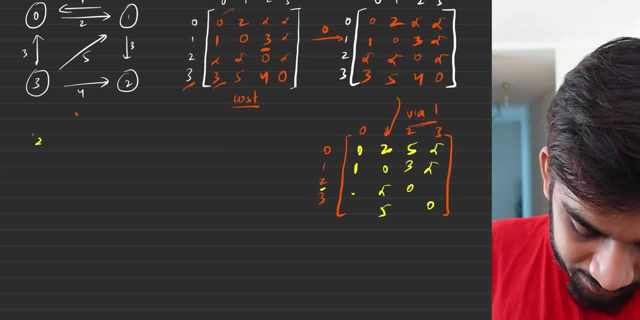 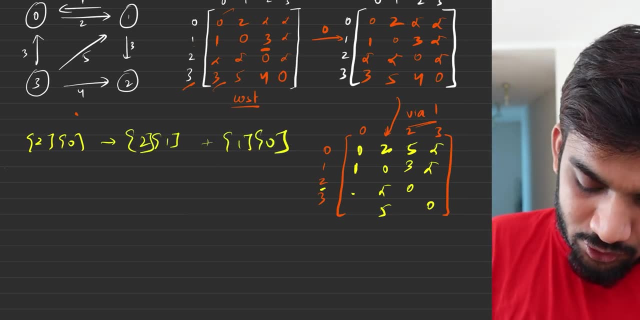 what's the next row? it's this one and this one: 2- 0. so if i go via 2- 0, that's going via 1, which is 2- 1, and then going from 1 to 0. let's see the values: of 2- 1. 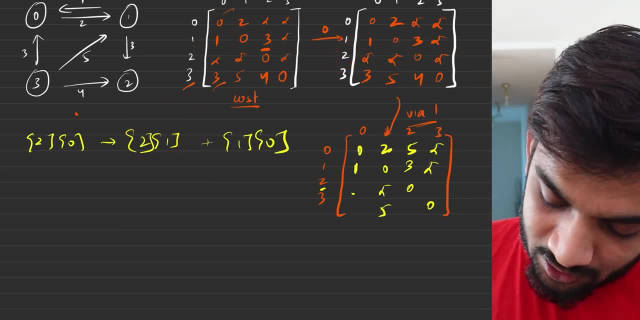 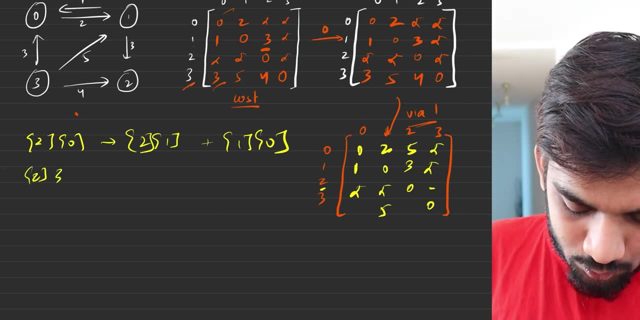 so i go 2, 1, infinity not to be considered. so, whatever is the value, just copy paste. still, we figured out. next is this one which is 2, 3. so if i go via 2, 3, which will be 2, 1 plus, yes, plus. 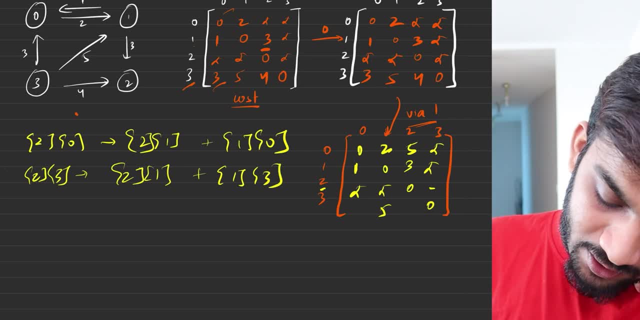 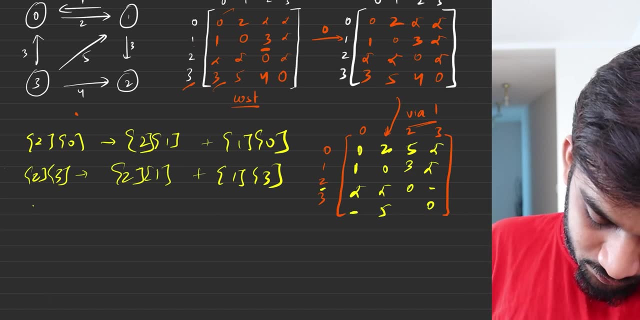 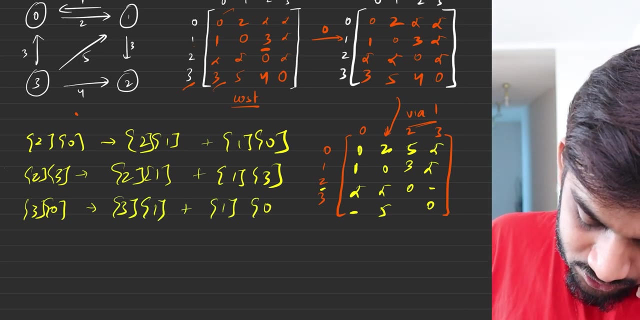 nothing but 1, 3. what is 2, 1? let's see 2: 1. infinity, again not to be considered. next, this is the next one: 3, 0. so if we take 3, 0, that's nothing but 3, 1 plus 1, 0, correct? so what's the? 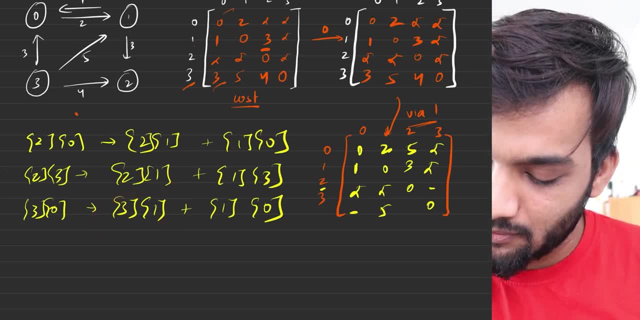 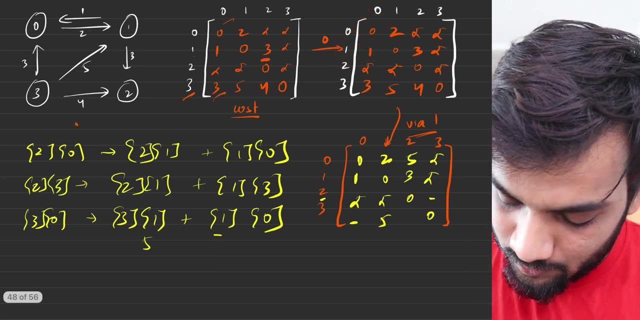 value of 3: 1. what's the value of 3: 1 guys? 3? 1's value is very simple: it's 5. so let's write 5 plus 1: 0. what's the value of 1: 0 guys? 1, 0 is 1, so plus 1, which is 6. so, as of now, what is the value? 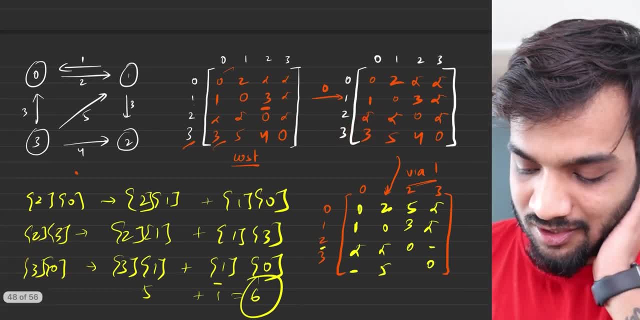 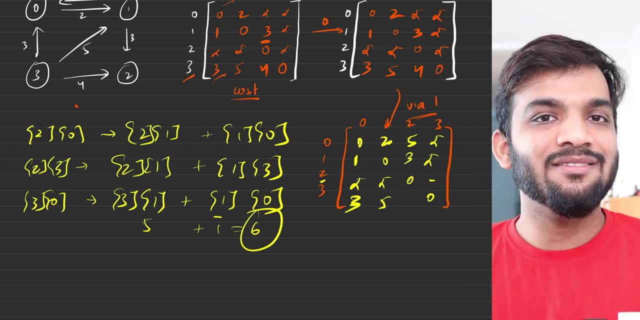 of 3: 0, it is 3. i'm already reaching 3: 0 at a value 3, so why will i take 6? so i'll keep reaching directly, reaching previously, whatever previous ways i've taken to reach 3. that's better, no need. 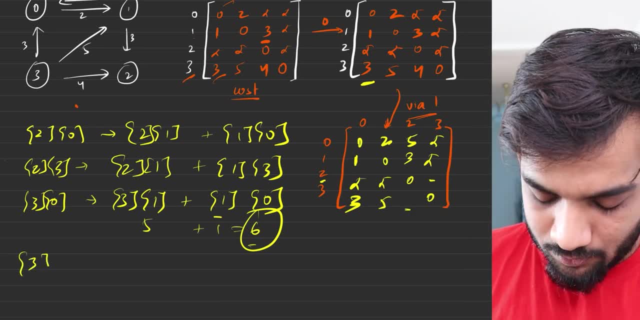 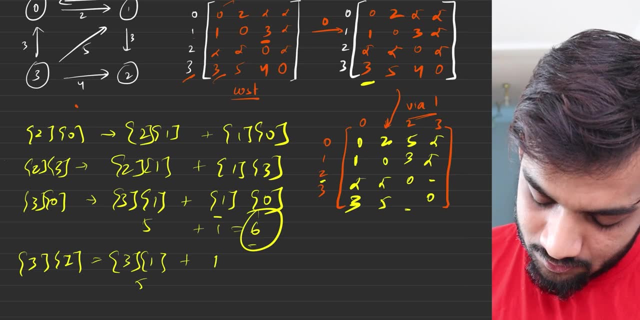 to take the new graded version. next is 3- 2. let's compute 3- 2. so if i try to compute 3- 2, it will be 3, 1 again, which will be 5, right plus 1- 2, which is nothing but 3. this time that's 8. so if you see, it's already. 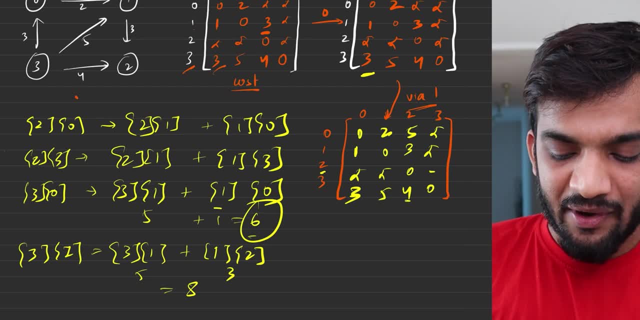 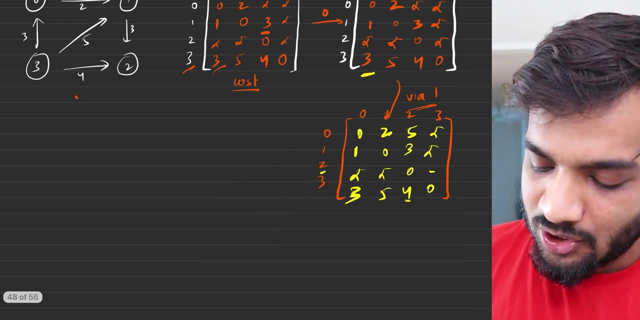 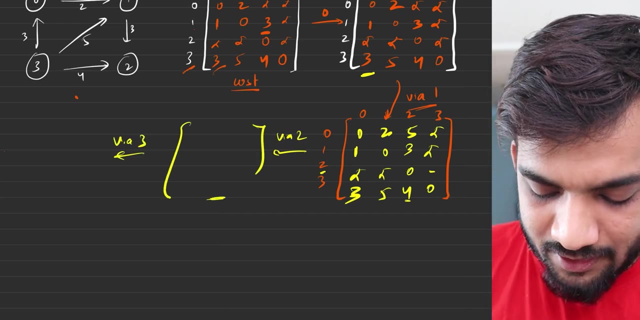 reaching at 4, so why will i take the 8 one? so, via one, i have computed it. i've computed the matrix via one as well. similarly, what you'll do is you will go via two and then you will get a matrix. using that matrix, you will do a via three and you will get an ultimate matrix. 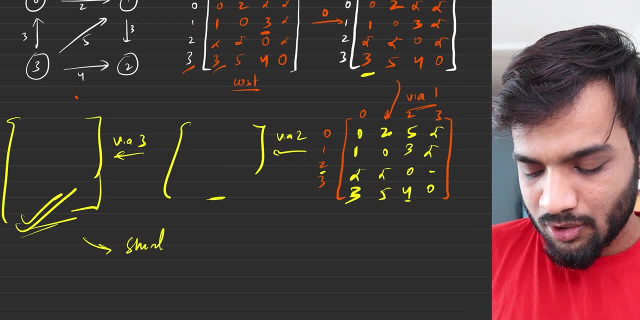 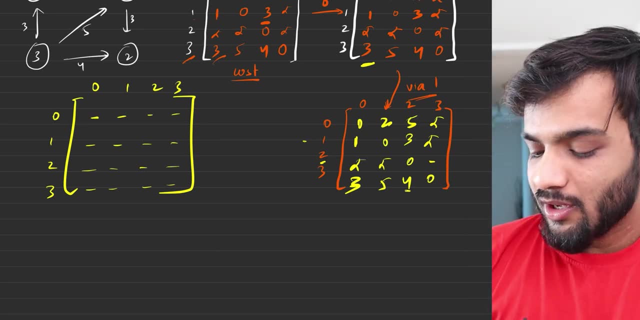 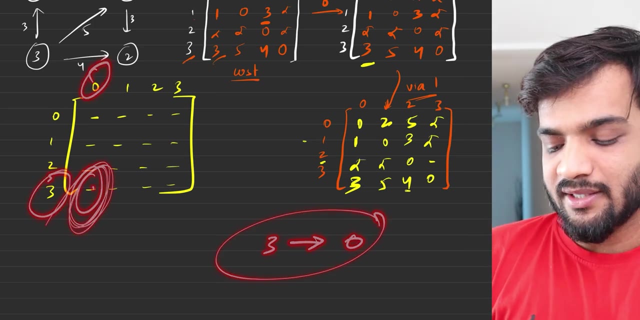 and whenever you get this ultimate matrix, this will be your shortest path between everyone, between everyone. so if someone tomorrow comes up and says you, hey, give me the shortest path between three and zero, so you go three, you go zero, and you say: whatever is stored here, that's the shortest. 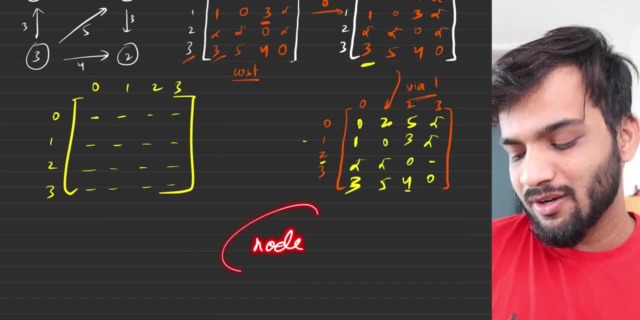 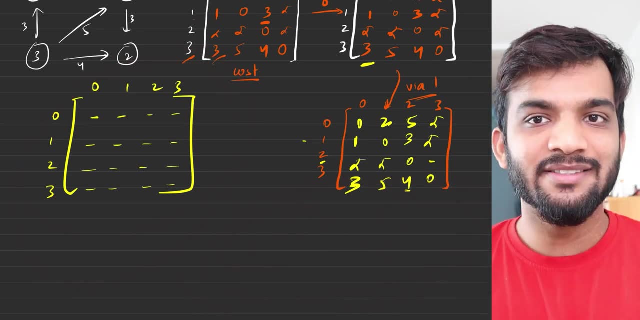 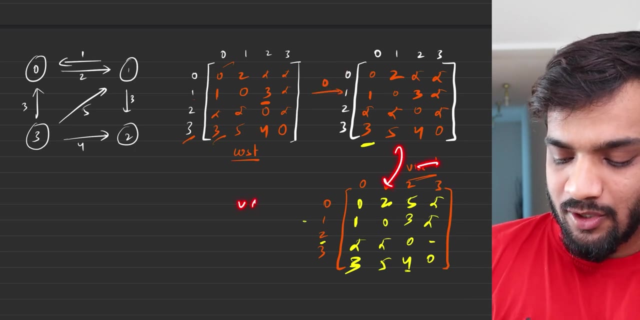 path so you can figure out, from every node one to every node two, the shortest path from this ultimate matrix that has been generated. so what are we doing exactly? at first we're going via zero, then via one, then via two, then via three. so can i say i'm going with everyone and whenever i'm. 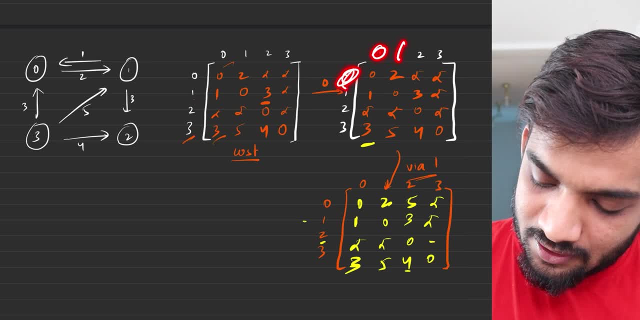 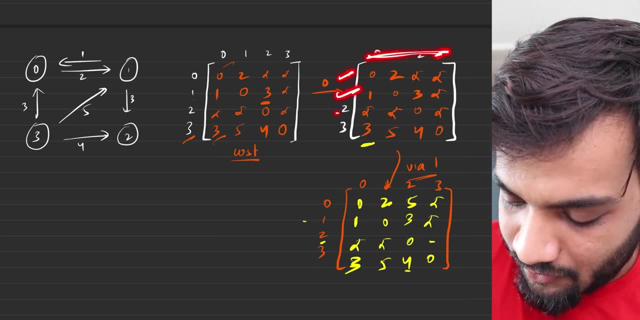 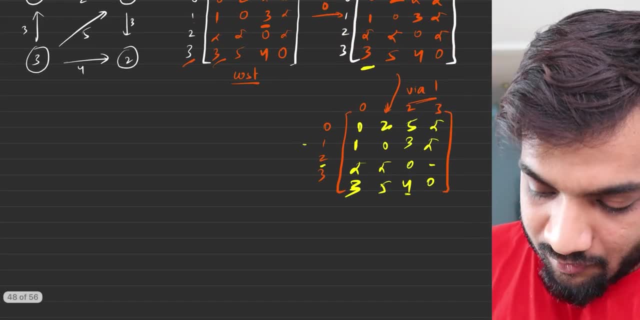 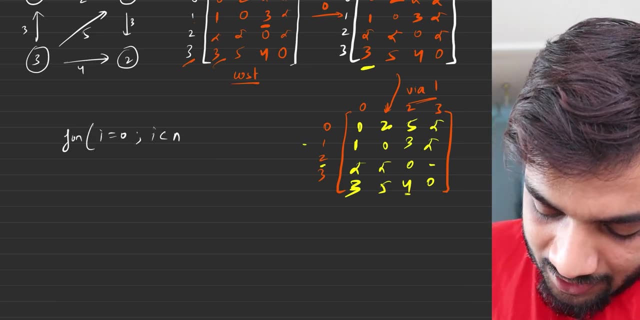 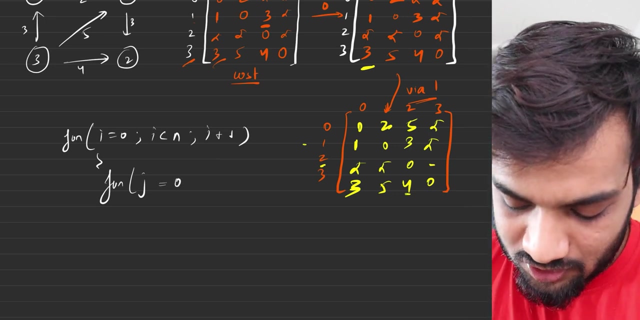 so in every iteration, can i say: what i'm doing is very straightforward and very simple and that's nothing. but i'm going from i, equal to zero, to the last node, and this is what i'm doing, because i want to go from i to j. so this is what i'm doing at every node. can i say this, yes or no? i can, and 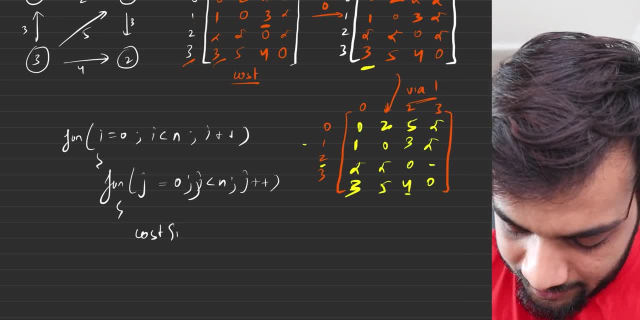 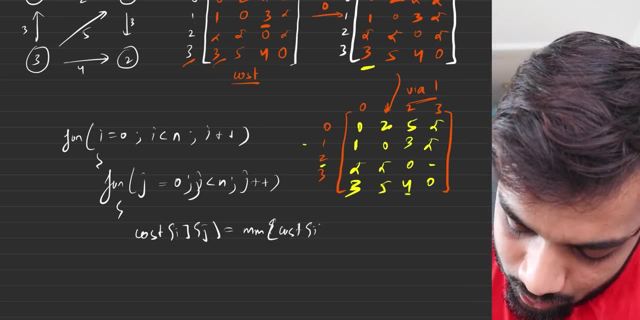 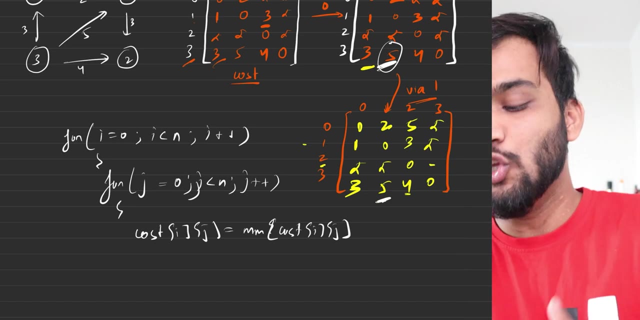 what am i doing? i'm trying to go for an example cost of i j. i'll take the cost as minimum of minimum of either what i have taken to reach it. that is currently what i'm taking currently. if i'm taking five, i'll consider that five and i'll consider the new one via one. so the new one via will be. 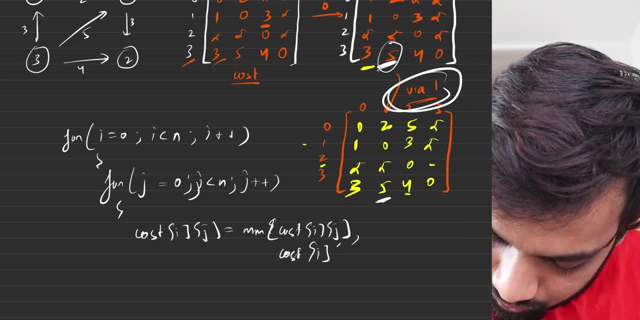 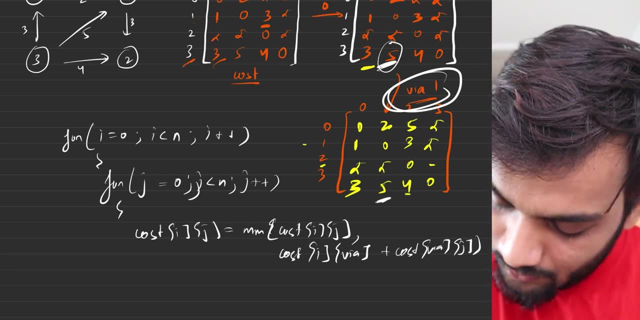 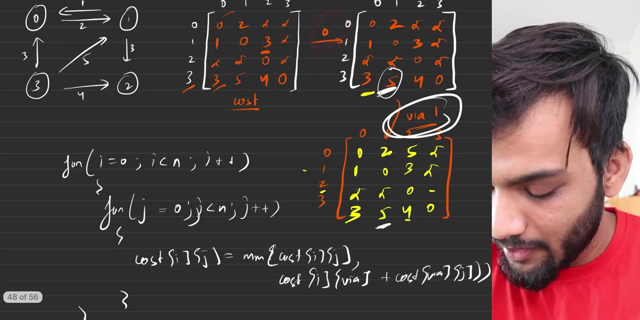 nothing but cost of i via, whatever you're going via, plus cost of that via of j. can i say this? i can and this is what i'm doing at every iteration, every iteration: first via zero. via will be zero here, next via one. so via will be one here, next via two, it'll get two. i'm trying. 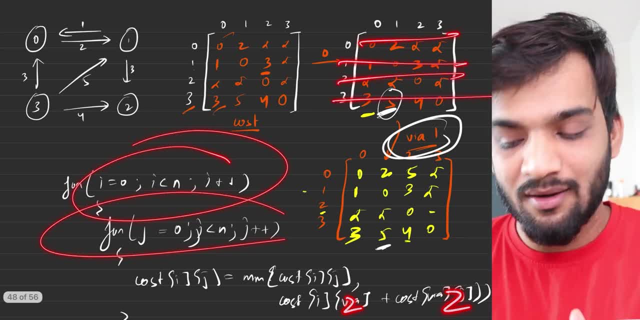 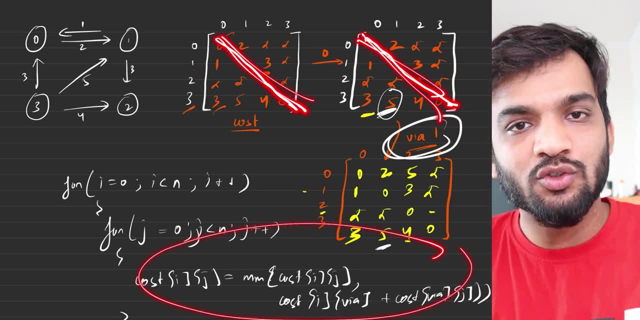 out everyone, trying out this, this, this, everyone, and automatically these will be zeros, because you have- initially, you would have- assigned zero, so this will take care that it will always be zeros when you do comparisons. so what is this via? first it is zero, then it is one, then it is two, then it is three. 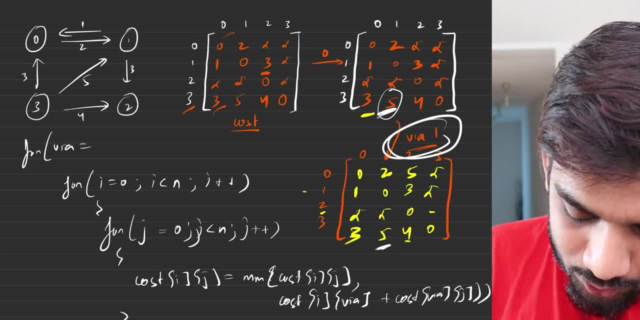 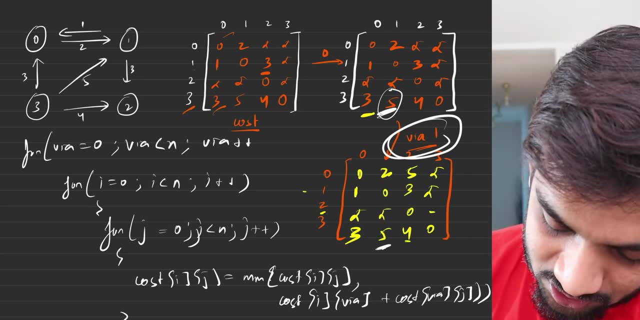 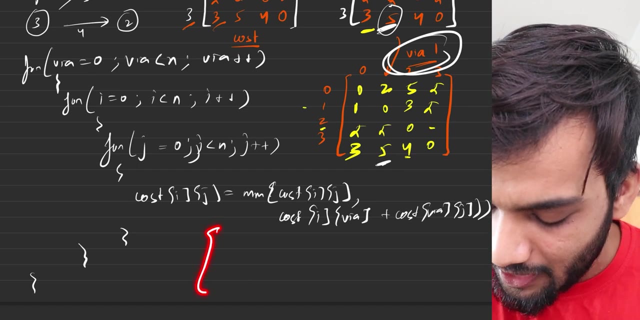 so can i say, for via equal to zero, via lesser than n, because zero one, two, three, every node till via plus. plus is what this will be, and once you have done this n cube loop operation, at the end of the day you will have your resultant matrix, which will be your answer. 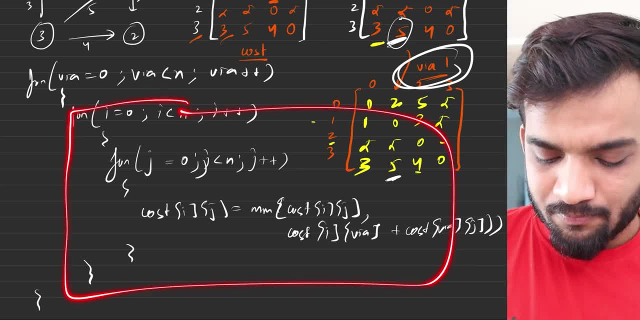 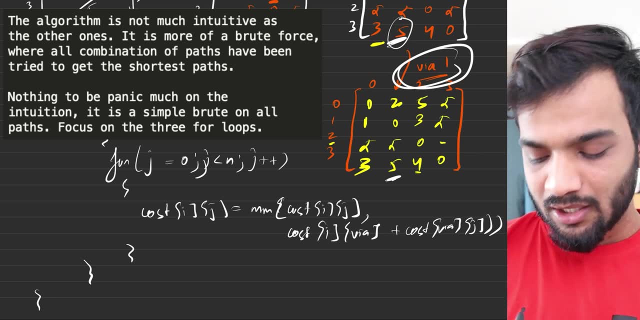 so, if you see, we have pretty much uh derived this one for every iteration and then we have wrapped it under a wire because via will always change. first get the via 0, via 1, via 2 and ultimately, the cost of IGA will be storing your ultimate shortest distance. 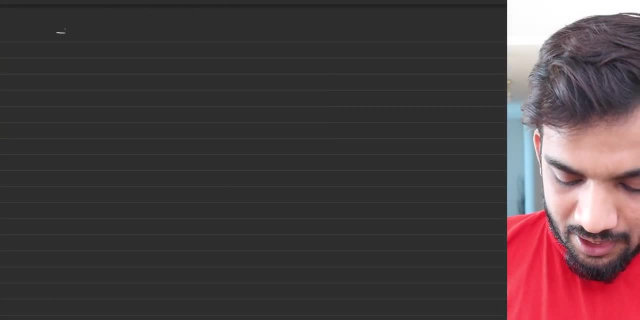 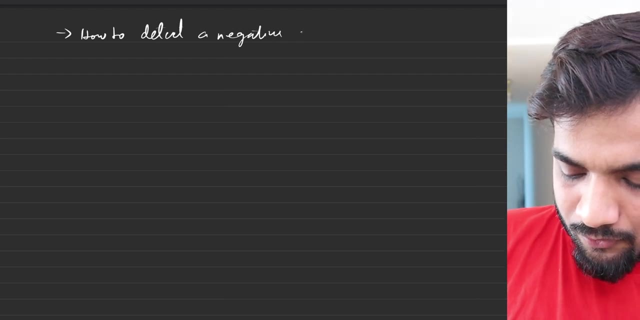 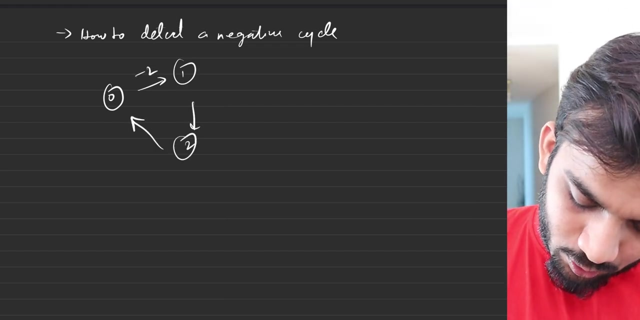 now couple of questions. first question is how to detect a negative cycle. what if the graph has a negative cycle, because we know for a negative cycle? imagine a cycle like this where we say: okay, it takes minus 2 minus 3 plus 2, so the total costing is minus 2 plus 2, minus 3 minus 2 plus. 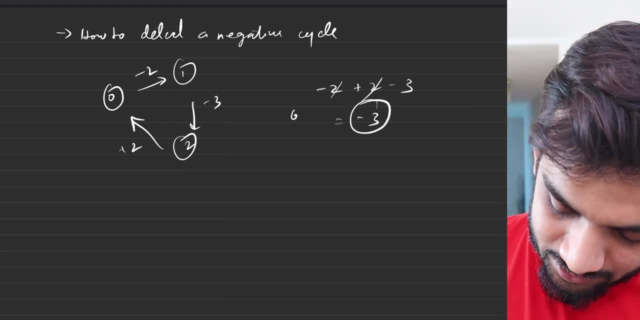 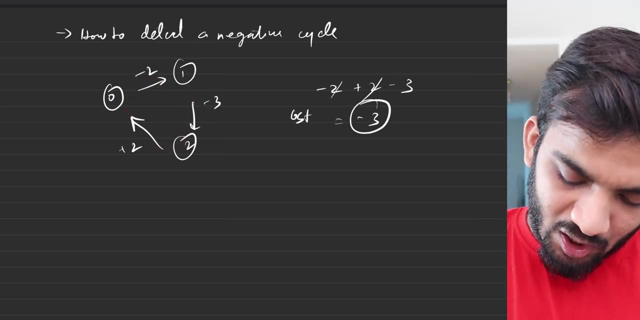 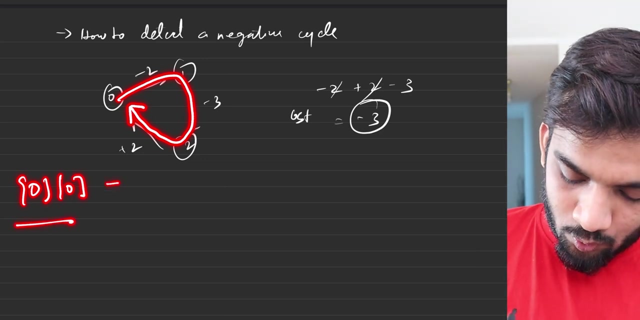 2 goes, so total costing is minus 3. so what will happen is the Floyd version will work properly and it will figure out a path via 1, 2 to reach 0, so the costing of 0 and 0 will be minus 3. 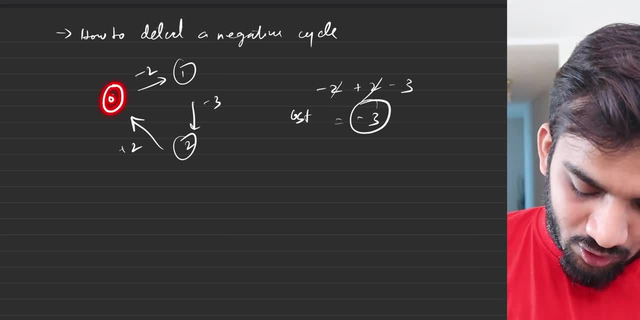 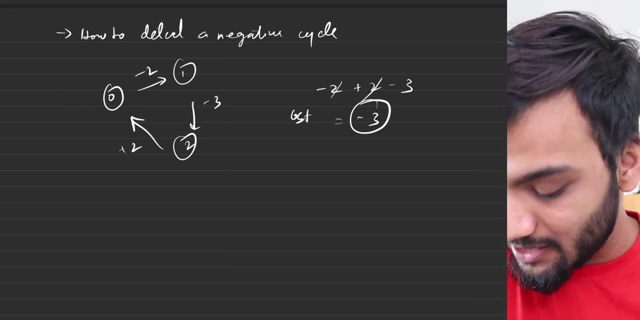 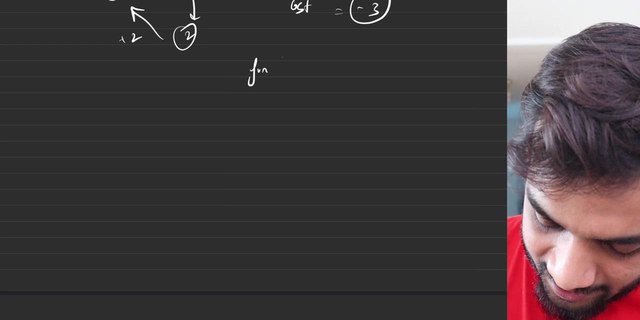 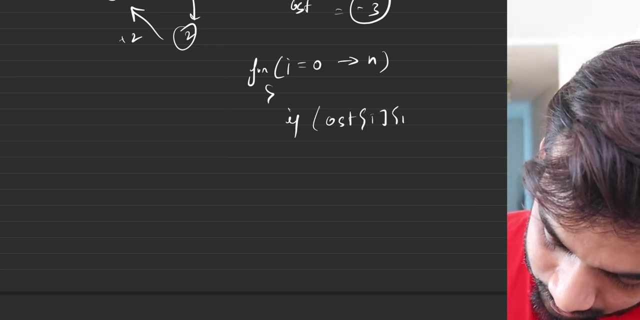 and apparently the costing of any given node to itself should be 0, because the node to node should always be 0, and if it is anything lesser to 0, if the costing of any node. can I say this: if the costing of any node from 0 to n, it's very simple. if the costing of I and I, which is the node to node itself, 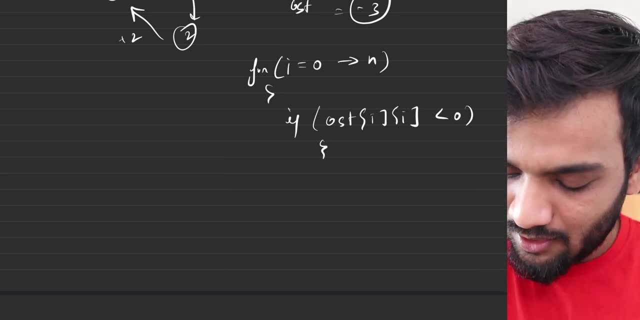 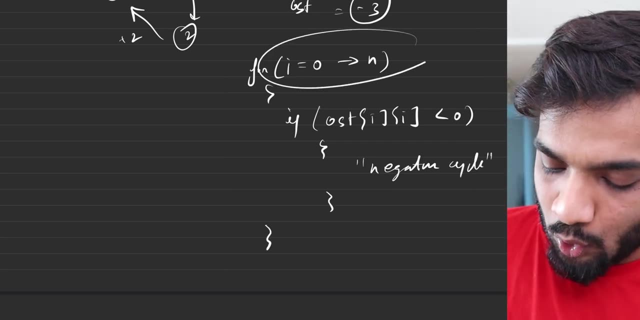 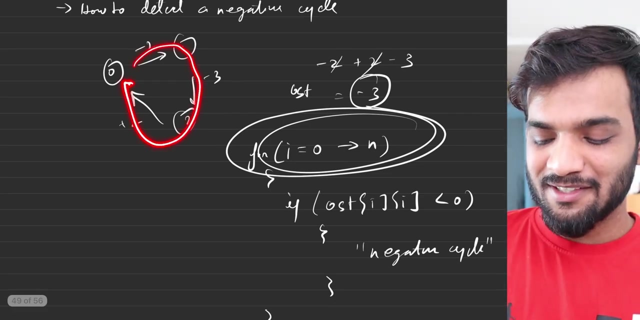 is lesser than 0, I can always say negative cycle exist. I can always say negative cycle exist. very simple: if we are going from all the nodes and node to node is less than 0 means flood. Rochelle has gone via this and has reduced the cost from 0 to something. 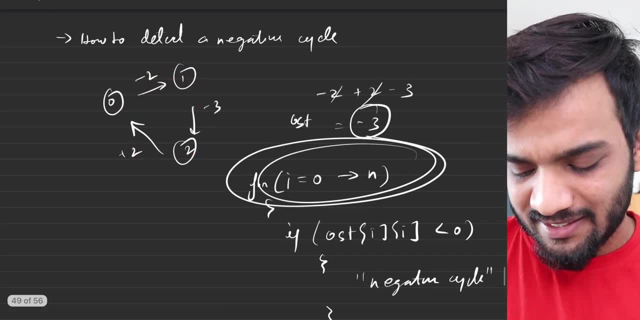 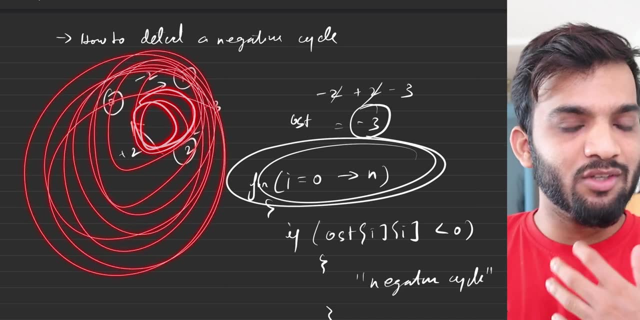 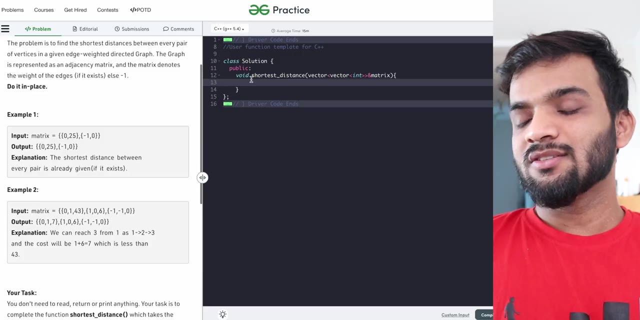 lesser because of a negative cycle. and you know, if it has a negative cycle it doesn't make sense to find the shortest path because someone will do unlimited turns and you'll just reduce it cost every now and then. so thereby it's not possible for negative cycle. so I hope you've understood the entire explanation. it's time to code it up so as 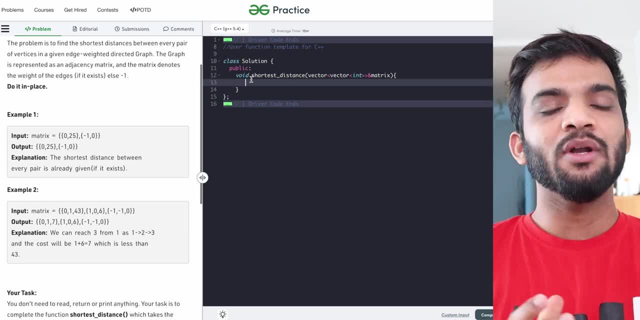 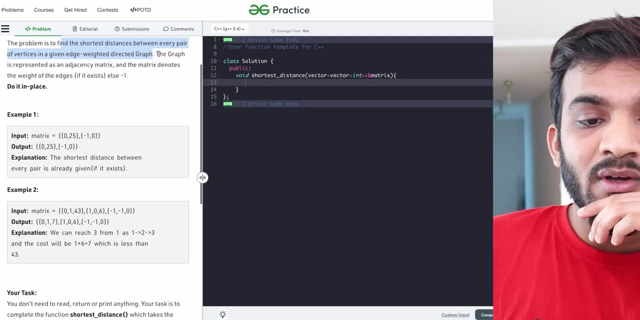 usual, the C++ solution is on the right and the exact similar java code is on the left, so you have to find the shortest distance between every pair of vertices in a given edge weight directed graph. the graph is represented by an adjacent matrix and the matrix denotes the weight of the edges, if it. 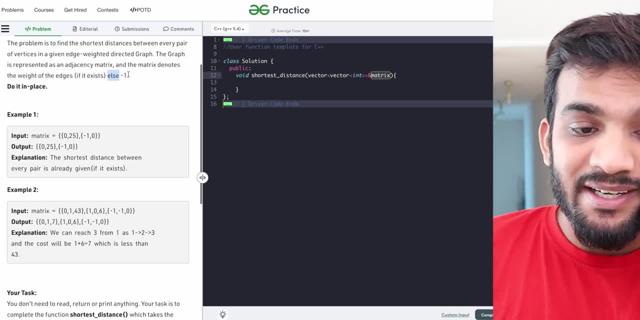 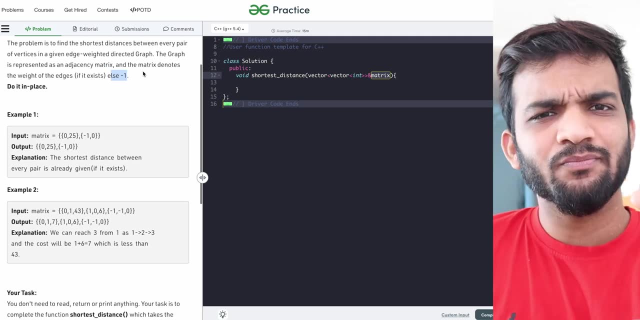 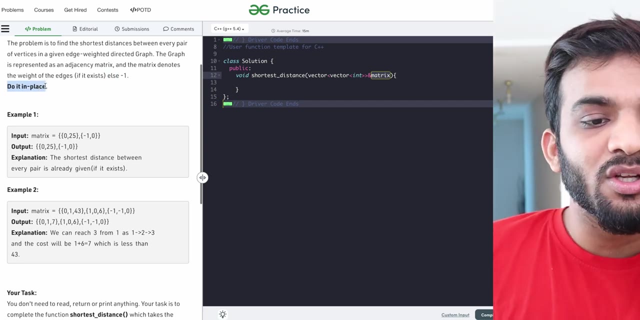 exits, else minus one. remember, they are stating minus one, not as infinity. if there is an edge, they're stating it as minus one. so you have to probably, you have to probably a bit of things before doing it. so do it in place. you have to do it in place is what you have to do and I'm assuming that there. 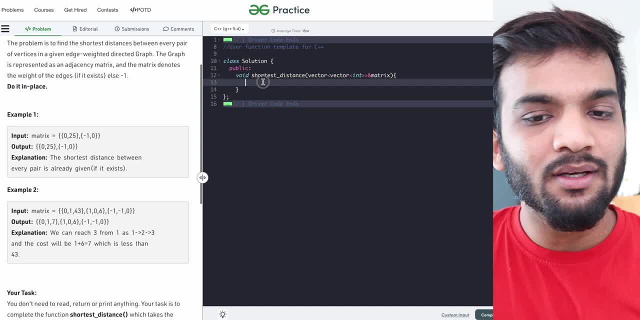 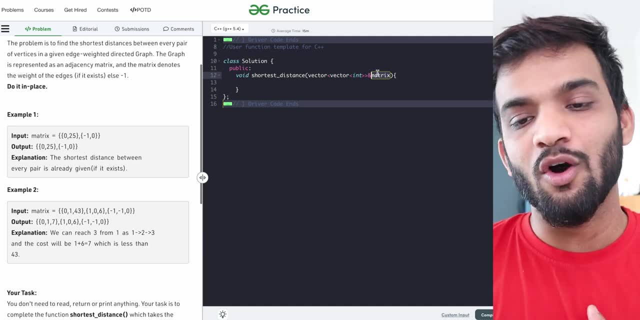 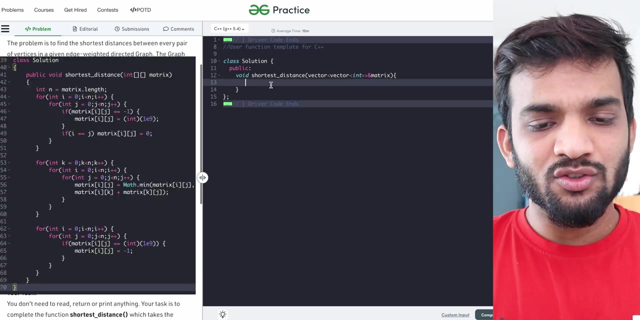 the graph does not contain negative cycles, otherwise they would have stated it. so you have to do it in place. we have to update it with the shortest book instead of actually doing a cost matrix and returning it. so remember, else minus one, so we not having to return it right now. this is our. 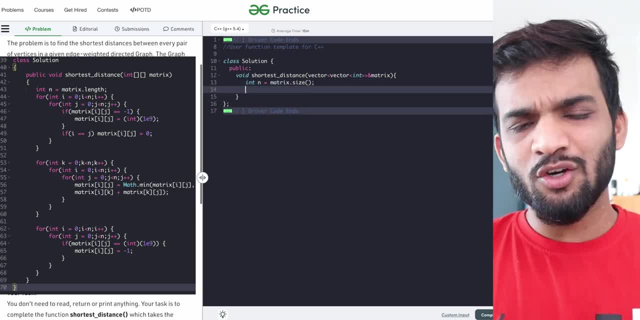 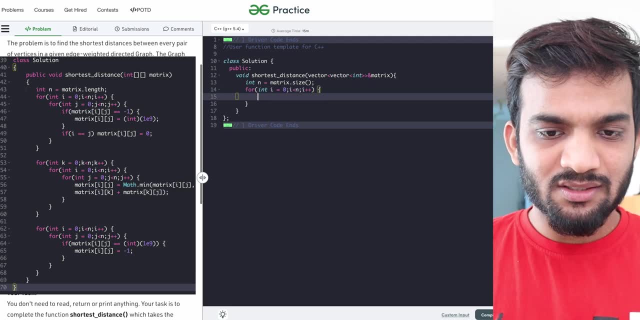 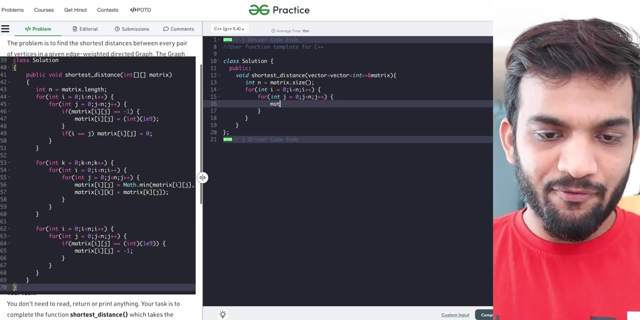 n at first. now, in in order to ease out understanding, what i'll do is i will just go across the entire matrix once, just in order to ease out understanding. you can avoid this step as well. so you can say: if, if, if, matrix of i, j is equal to, equal to minus one, which actually means 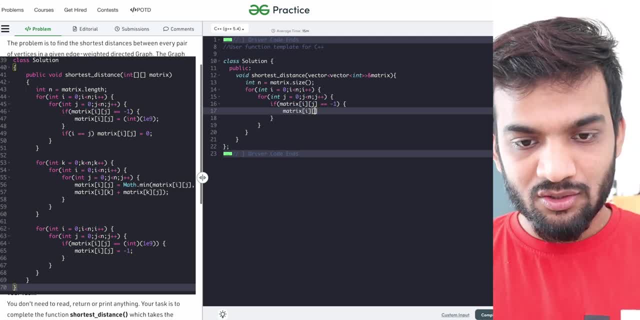 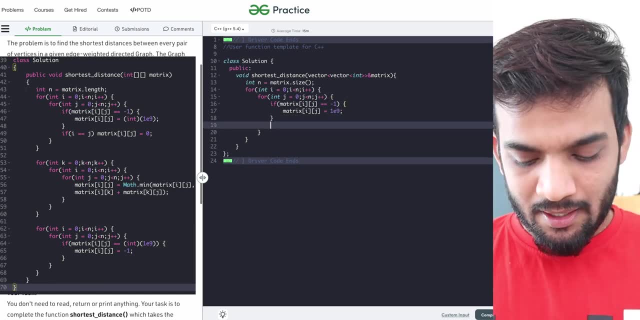 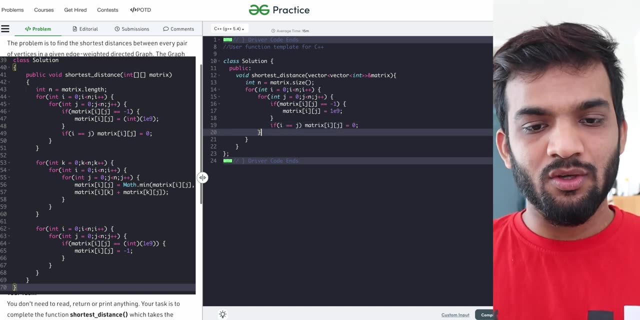 that it's not possible to reach it. so i can say one in and i'll just give it a very big value and while i return i'll just change it to minus one. and one other condition i'll always keep if i is equal to, equal to j, which is the diagonal. i know the reaching place is always zero, so that's. 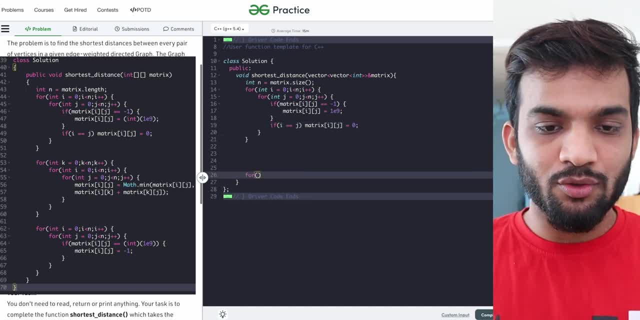 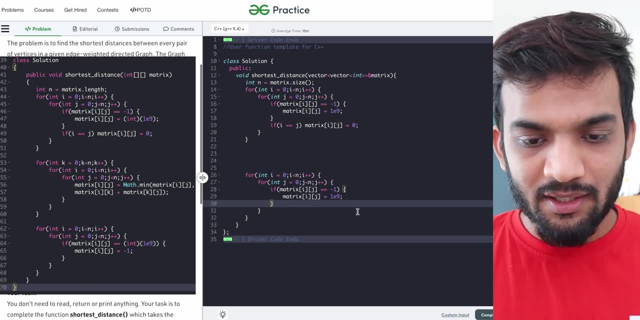 what i'll initialize and, before returning, just make sure you do the same thing. yes, before returning, just make sure you do the opposite of it, okay? so before returning, if it's one in, i j. it's not possible to reach it, so i can say one in and i'll just give it a very big value. 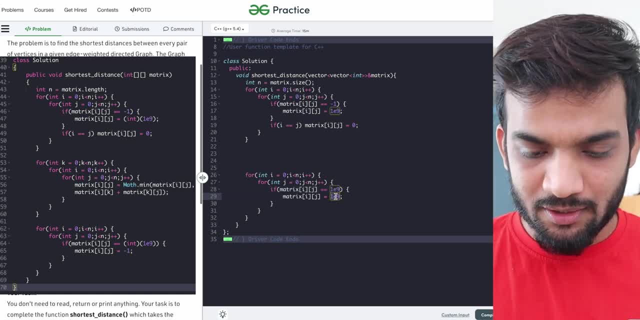 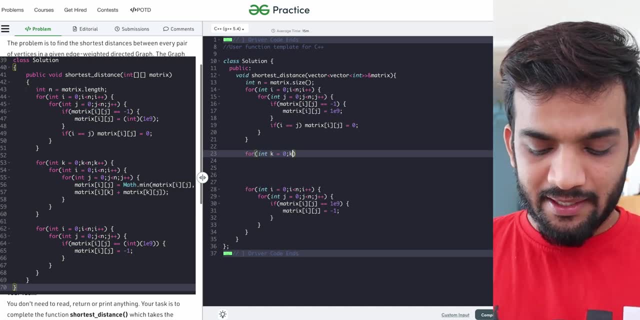 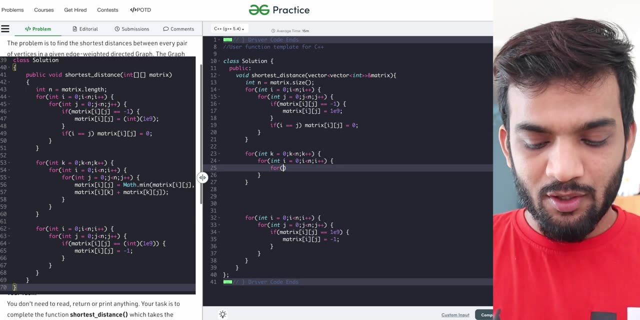 still, which means it's not reachable. and if it's not reachable, do it a minus one before returning. you do this, okay. now let's perform our algorithm. it's very simple. we know k will be zero and k will go till less this and after that, we know i will be zero and i will also go till this and we. 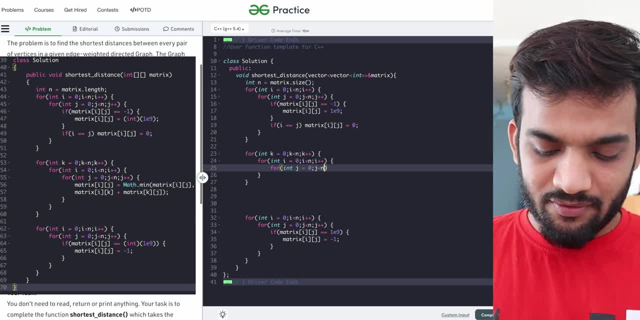 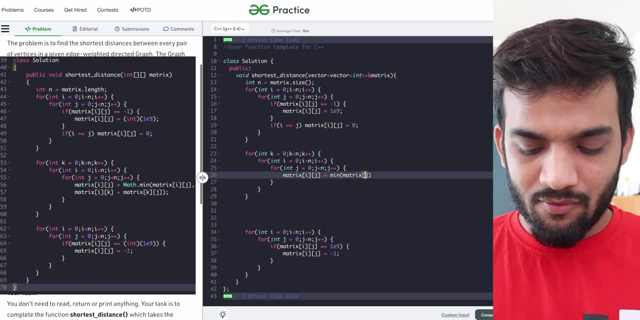 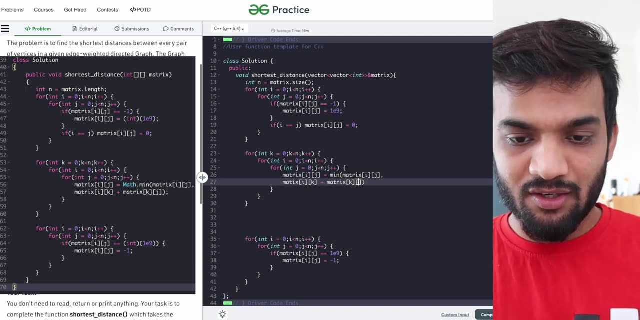 know the other thing will be j equal to zero and j will go lesser than this and the uh other thing we know is matrix of i. j will be minimum of matrix of i, j comma, you matrix of i via key, so this, and matrix of k to j and i think this should be more or less. 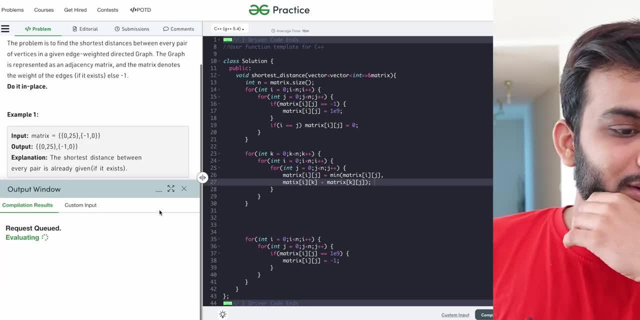 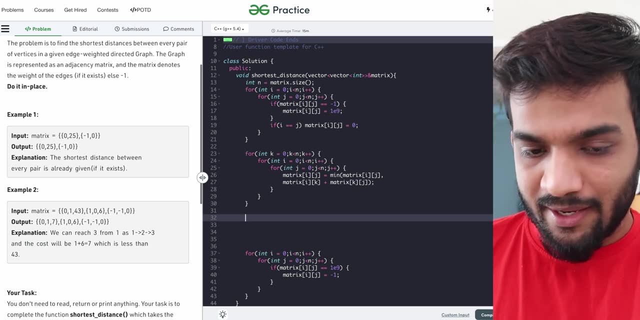 it about the algorithm. it's a very uh straightforward one. so if you see, on compilation it is giving the correct output, so i'll submit it and, yeah, it does pass. so one more thing to add before i wrap it up. if in an interview someone does ask you what if there is a negative, 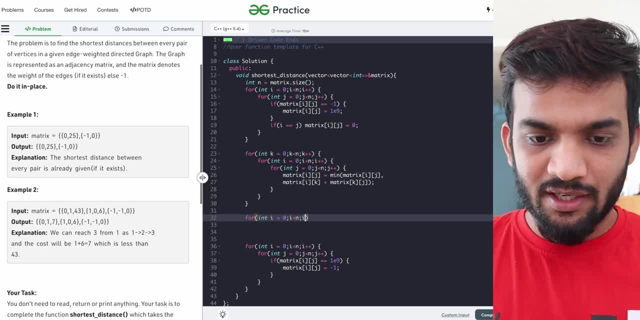 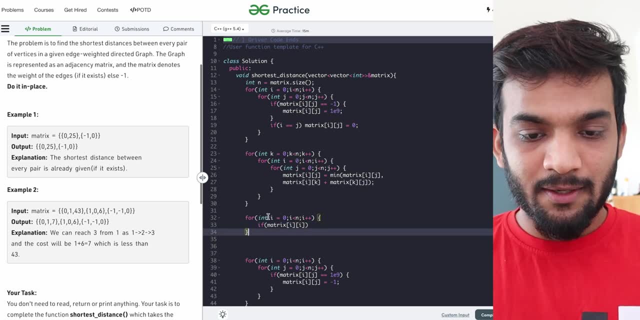 so you'll say, hey, i'll just probably write something like this over here. if it's a negative cycle, i'd be like, if the matrix contains i, i lesser than zero, before assigning this lesser than zero, then i can probably print something or something like this: i can do it over here. 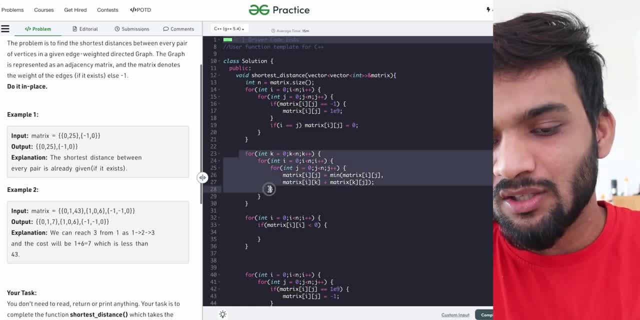 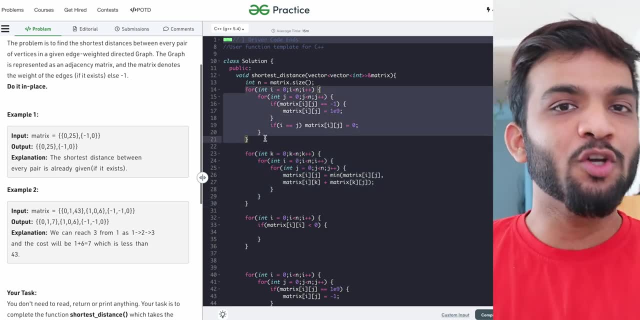 so let's discuss the time and space complexity. the time complexity of the algorithm, major time complexity is n cube, definitely. now a lot of you will be thinking the space complexity is big of one because you're using the given matrix. no, whenever we talk about space complexity, it's. 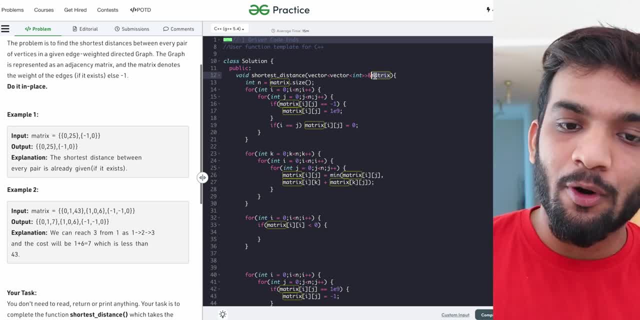 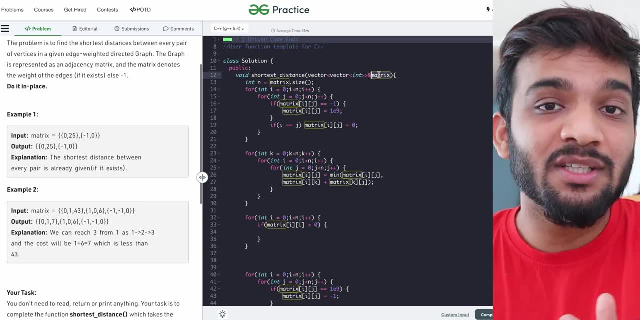 generally the space that i'm using to solve the table. when we think about the quantity that the unused space tab has, the specialized x that I'm using to solve the problem. in order to solve this problem, I'm using matrix, so that is the space that I am using. if I would have not been using 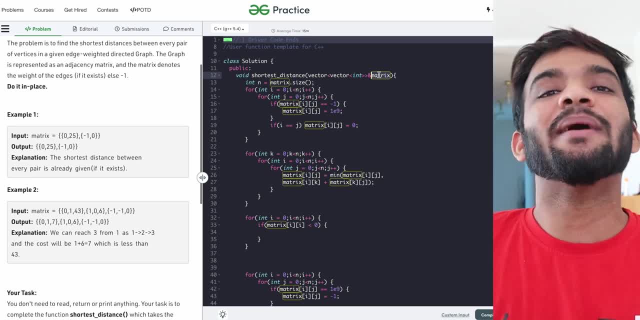 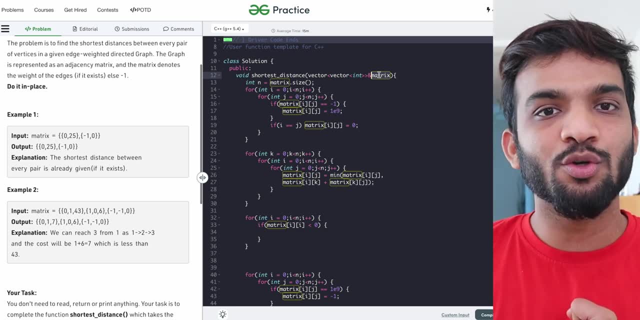 this, then I can avoid it. but if I'm using that goes inside my space that I've been using. I'll say: the n square is the space we're using, a cost matrix. the cost matrix will be your space, which is n square. you can't see if someone is. 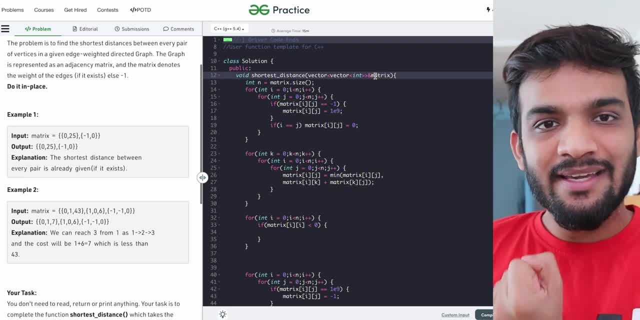 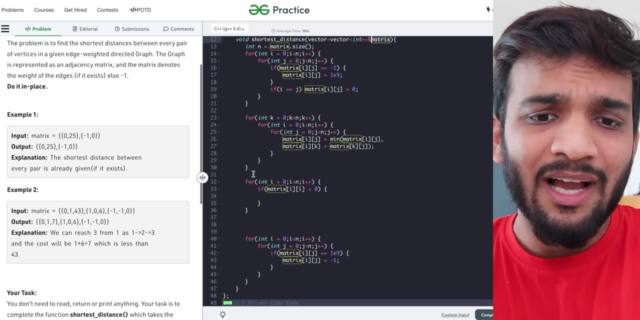 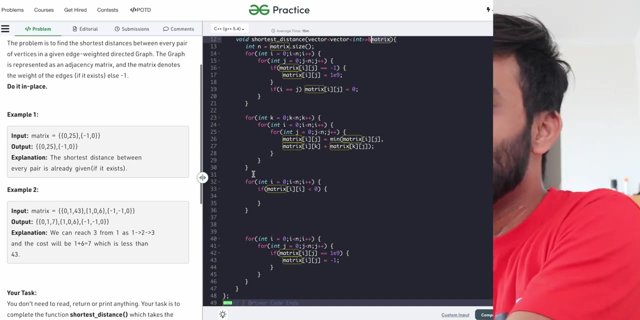 giving you something. it does contain a space. we're taking it. you need place to store it, right? so you are using some space which is n square over here. so I hope it is clear. I might be thinking: but, Shriver, what if you'd have implemented Dijkstra? so let's go back and analyze that as well. so if you remember Dijkstra, 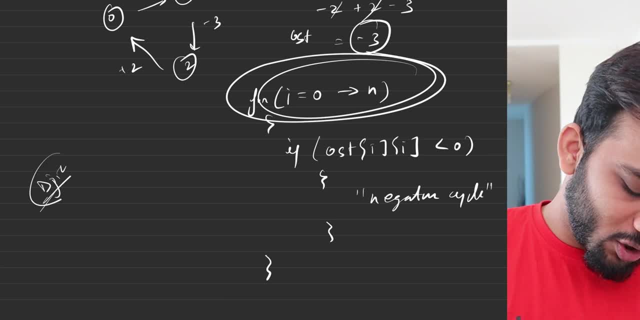 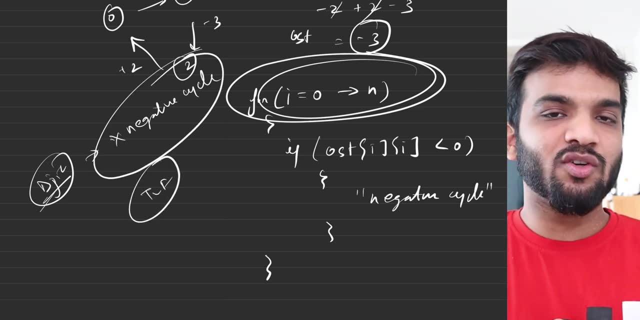 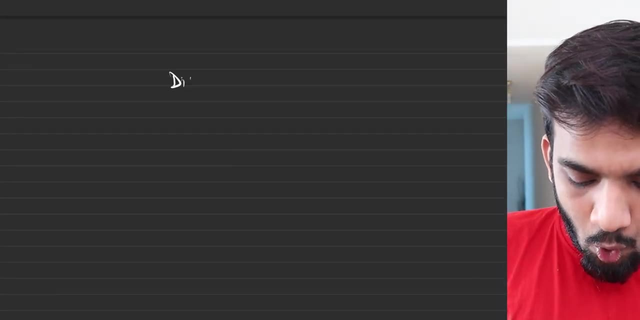 does not- yes, does not works for negative cycles, it will fall under, yes, a TLE loop. so that's where Dijkstra cannot be implemented. but if the graph does not have negative cycles, then it doesn't work. because the graph has negative cycles or something, you can actually apply a dixtra for all the nodes, because dixtra 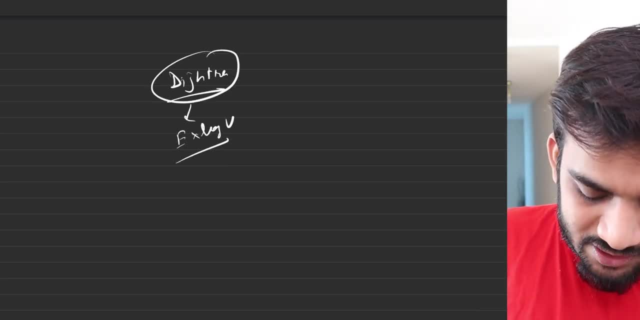 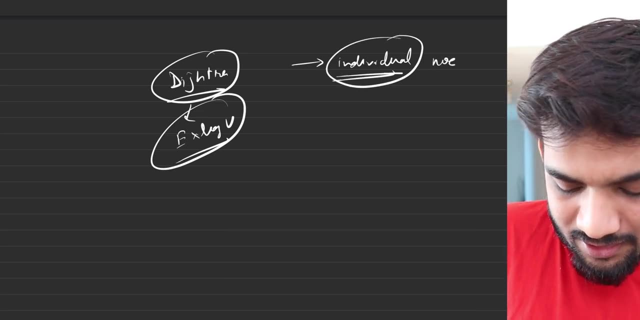 in itself takes e log V. so what you can do is apply dixtra on every individual node to find out the answer. every individual node, and there will still be n cross e log V, so it'll still be less like V cross e log V. it won't go. 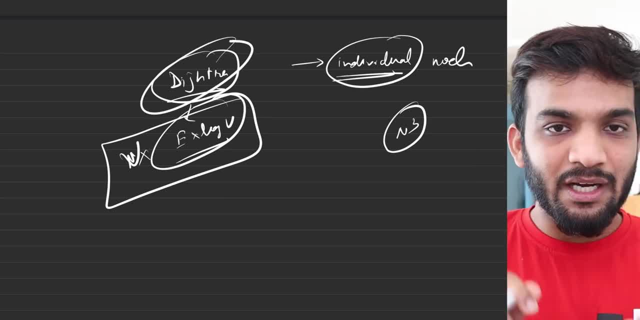 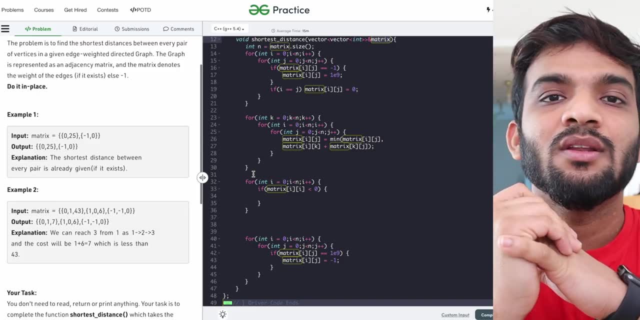 till n cube which the fluid ocean is taking. apply individual dixtra on every node to get every pair distance. you can do that, but it doesn't work for negative. now if in an interview someone does ask you about fluid ocean, do not just tell the algorithm. tell about these extra things like: why does something like a 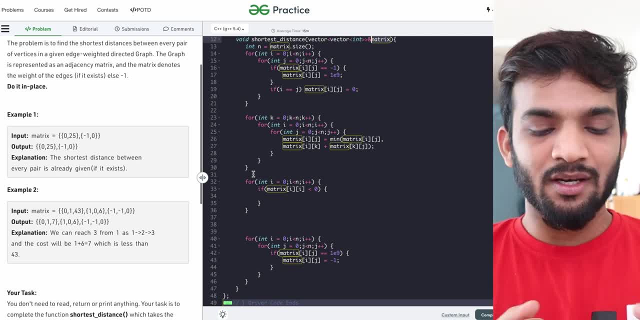 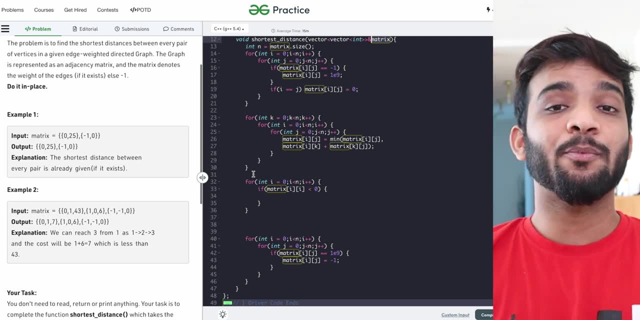 dixtra will not work where. how can you detect a negative cycle if you add up these extra points in an interview? it's always a cherry on the cake, so make sure you add these extra points if the interviewer does ask you about the fluid ocean algorithm. so, guys, I hope I was able to explain you the fluid ocean. 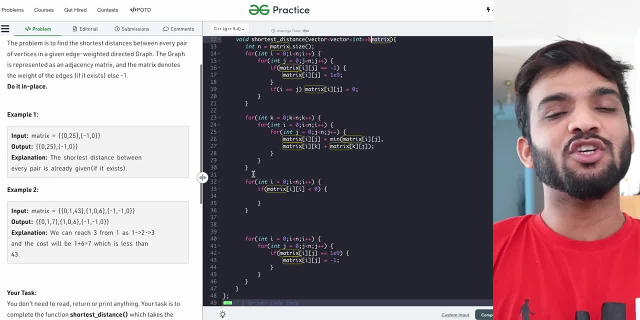 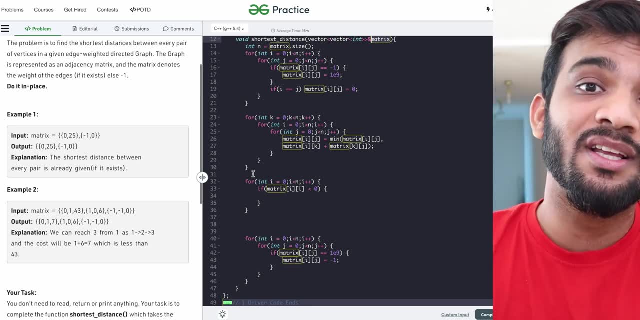 algorithm. you and you've understood everything. just in case you did. please, please, please, make sure you like this video and if you're new to our channel, what are you waiting for? I think it's time that you hit that subscribe button and if you haven't checked out our dp series and the HDC, the links will be in the description. 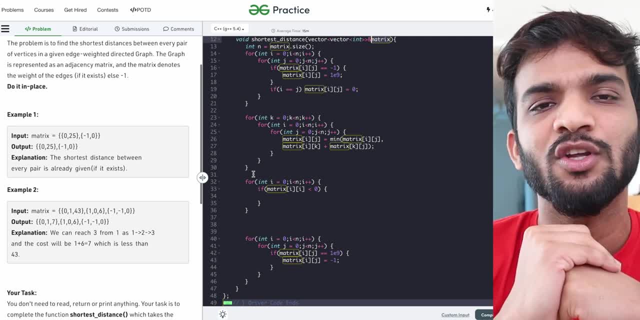 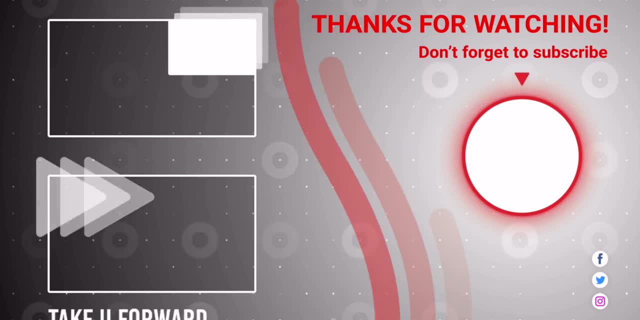 please make sure you check them out. with this I'll be wrapping up this video. let's meet in some other video. till then, bye, bye. take care: whenever your heart is broken, don't ever forget your golden. I will find a light.